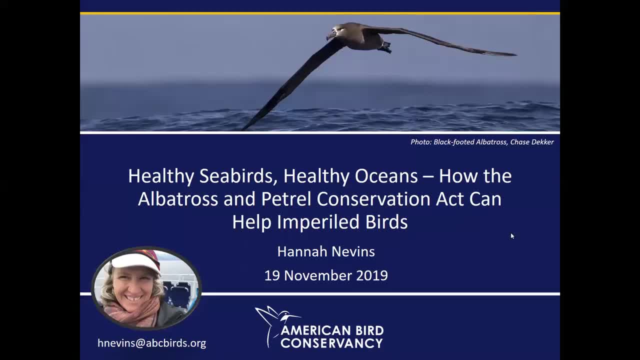 So good afternoon. I'm calling from Santa Cruz, California, where I'm based along with Brad Kitt who, as Jennifer mentioned, is our Oceans and Islands Director. So I'm happy to be talking to you today about some of my favorite birds and kind of bridge this gap between the conservation and the science with the policy actions. 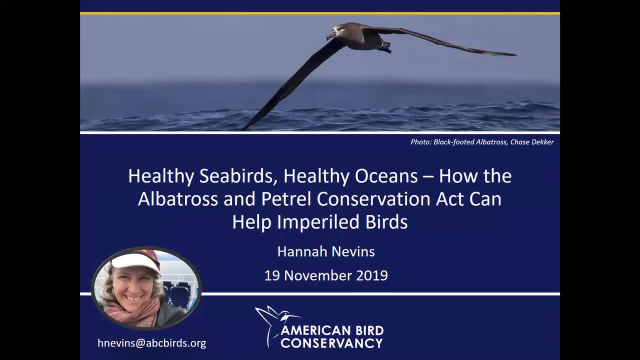 And I think the Albatross and Petrel Conservation Act is a pretty critical act for many of the species I study and the 146 global species of concern. So I want to just take a minute to tell you where my history with these birds starts, since my screen will allow here. 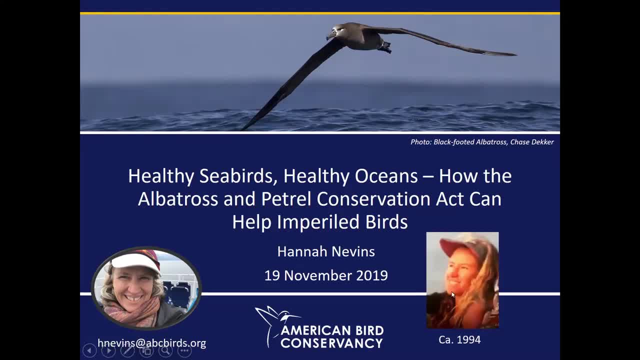 So there's a picture in the right hand corner Of me in about 1994 on Laysan Island, when I first met these birds, like this black-footed albatross pictured in the Laysan Albatross pictured, And little did I know that 25 years later I'd still be talking about these birds. 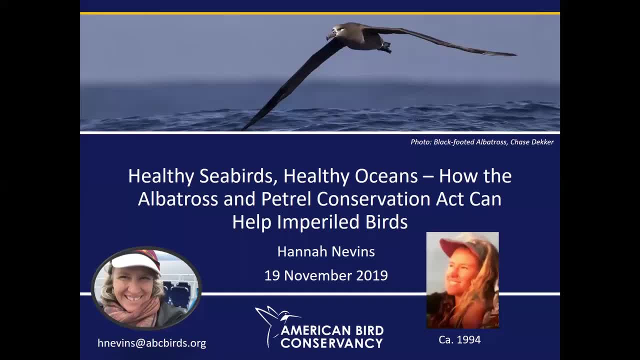 And also what's astounding to me is that many of the birds that I met on the island that summer are still living today. So these are really long-lived birds And are still alive And our lives are sort of parallel in that way. 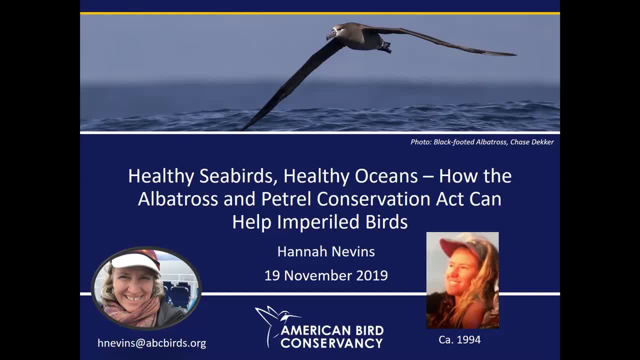 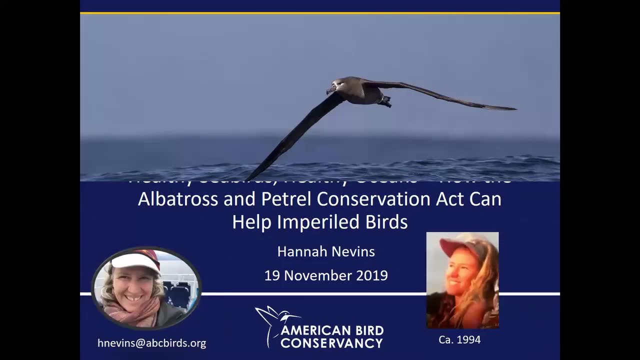 I've also, just as a note, I put my email down in the left-hand corner, So feel free to reach out to me if you have additional questions or follow-ups on this webinar. So interestingly you know, my journey with the albatross began in the mid-'90s, as did the American bird conservancy season. 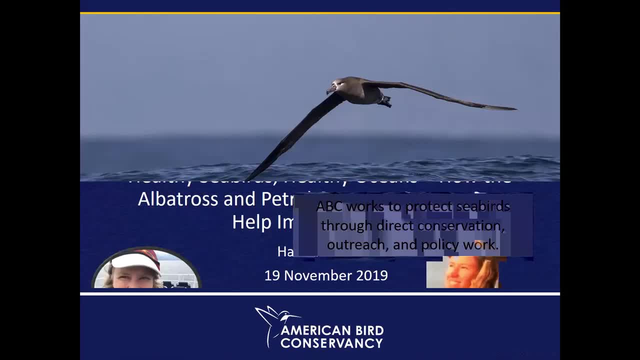 ABC, as it's known, works to protect seabirds through direct conservation, outreach and policy, And it was really in the mid-'90s that the effort in industrial long-line fisheries was ramping up in the middle of the Pacific and brought a call to action for ABC and other bird conservation organizations to really address this issue. 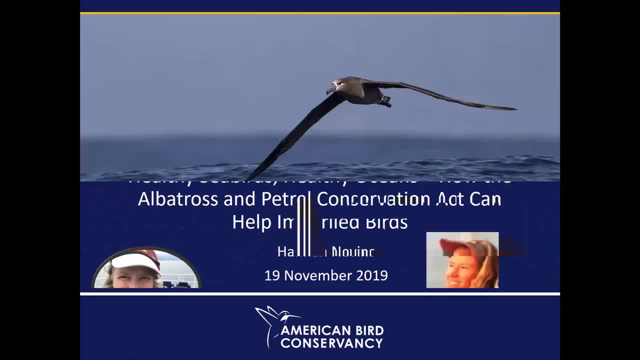 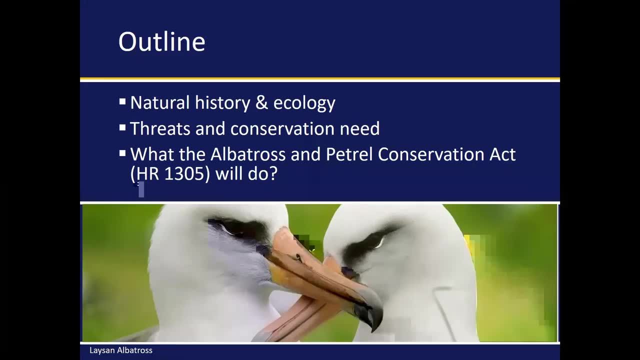 And so I'm going to talk a little bit about the movement, And so I'm going to talk a little bit about the most direct threats. But first I want to just introduce you to some of the species and their natural history and ecology. 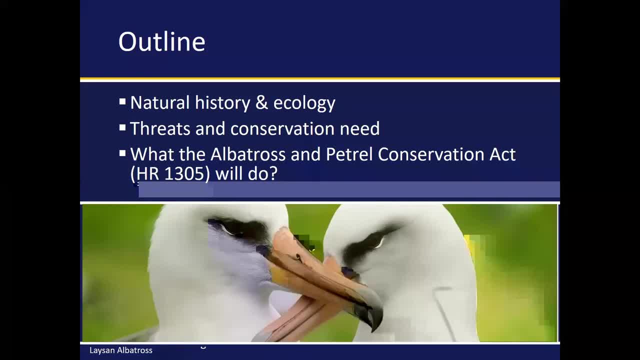 And then get into the threats and conservation needs And then more of the specifics of what this Albatross and Petrel Conservation Act- or HR 1305, as it's known in the US- will do. So at that point I just want to stop and make sure everybody can hear me. 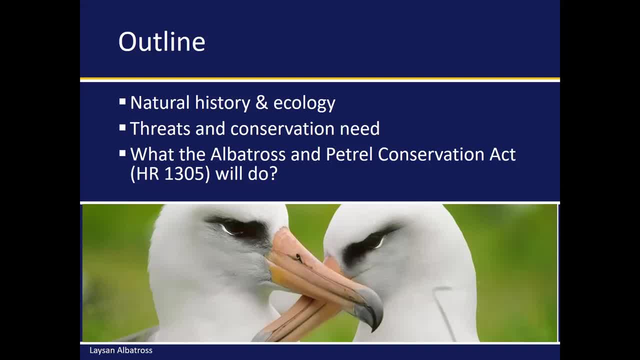 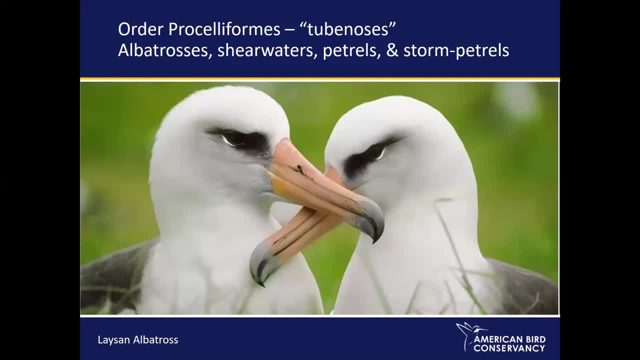 Okay, Any audio issues? Jennifer, Everything going all right? You sound great, Hannah, Okay, Okay, Good Thanks. So the albatross, shearwaters, petrels and the small storm petrels are all part of the order of prosolariformes, or the tube noses. 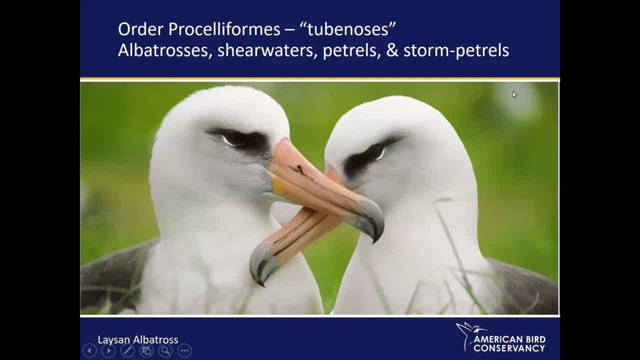 And so they have this characteristic feature on the top of their bill, which is the external opening for their nose, And that does that. It gives them this really keen sense of smell and also helps them in navigation, And so that's a feature that distinguishes them from the closely you know resembling gulls, salarids and skuas. 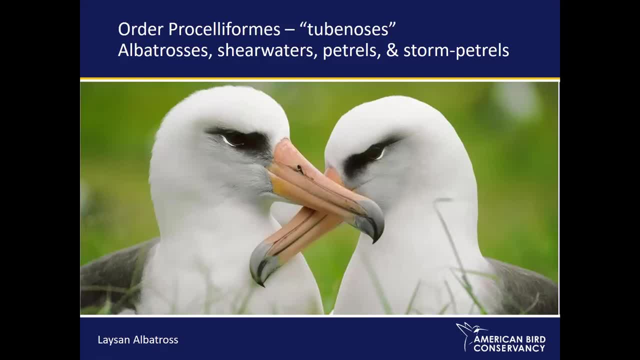 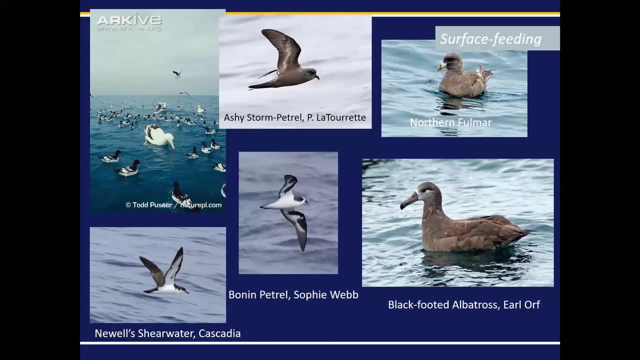 But these guys have a very different morphology. So here's in this next slide, a picture of some of the diversity of the prosolariform seabirds. So there's four families: the albatross, the petrels and shearwaters. 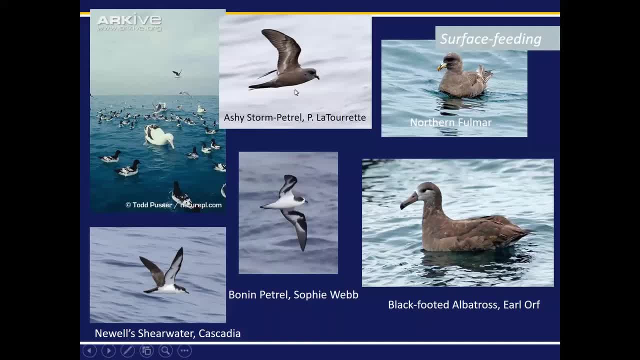 And then there's two families of storm petrels And for the most part the act covers the majority of these species, And storm petrels have yet to be added to this list. So these are primarily surface-feeding birds And you can see in the upper right, the northern somar has this really exaggerated tube. 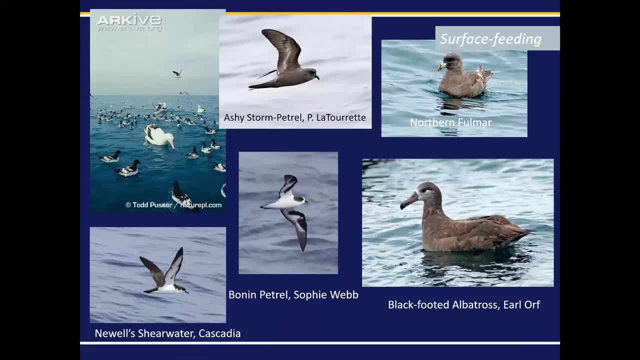 It almost looks like a drinking straw on the top of it And these guys have a really great sense of smell for locating prey across the vast ocean. And also it's thought that they use that sense of smell to hone in on their colony so they can smell colonies from great distances. 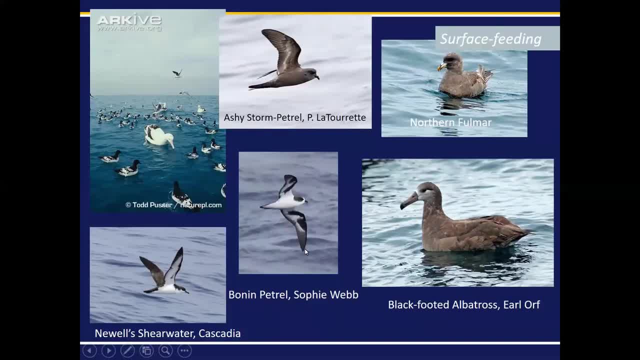 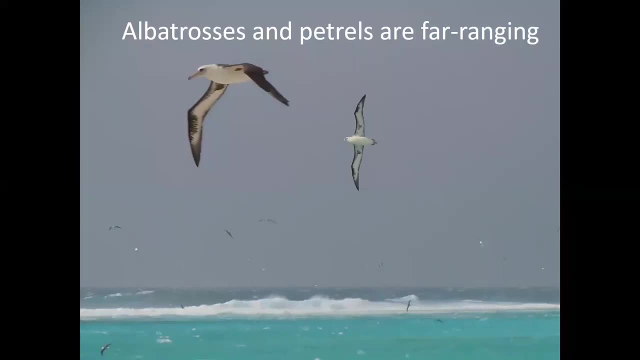 You'll also notice in the omen petrel, in the center they have these real long tapering wings And that enables them to traverse the ocean, And that allows them to traverse large areas of the ocean with very little energy. So here's the Leysan albatross. 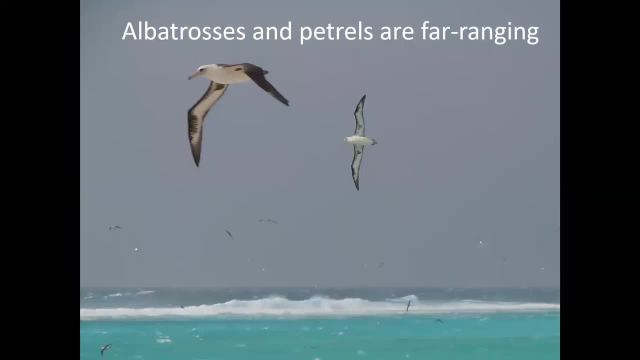 They're very far ranging. The Leysan albatross has a range of about 49 million square kilometers, So try to wrap your head around that number. They're traversing huge areas of the Pacific And, again, the way that they do this is they have real efficient design. 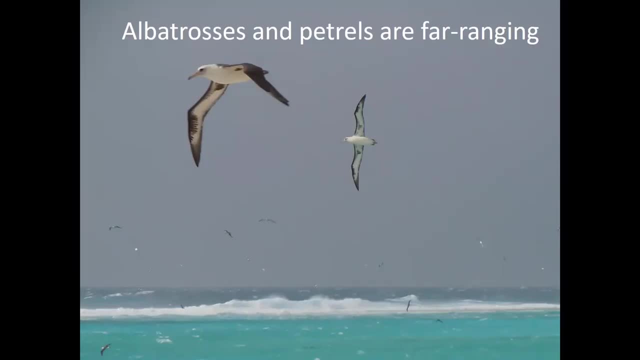 So it's quite spectacular to watch them in midair in high wind speeds, as you see in this picture, where their wings are just straight across- And this is about a seven-foot wingspan And there's not much flapping flight at all- as they use the wind's energy to make a sort of a figure-eight sort of pattern as they move up into the wind current. 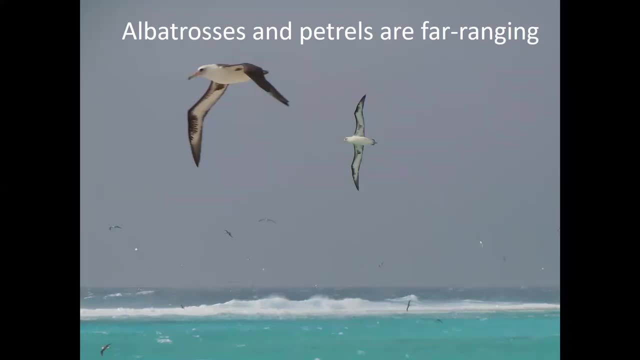 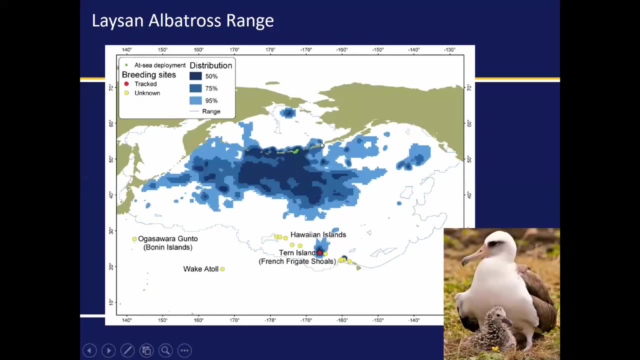 So this enables them to move great distances with very little energetic cost And, as a result, we see that this is the range of the Leysan albatross here. So just to orient you, the continents are in kind of this grayish-green color. 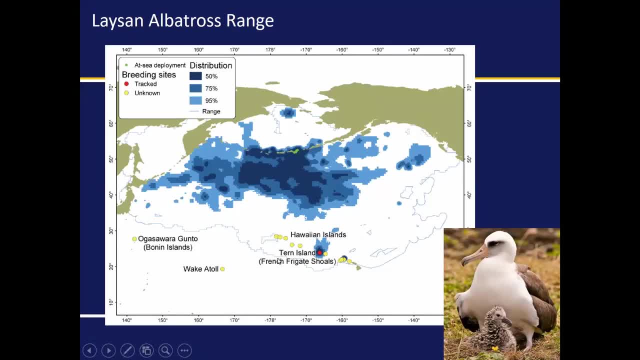 And you can see this dotted blue line that starts around French Frigate Shoals and goes extends to British Columbia and over to Japan. That is the range of the breeding birds tracked by satellite from Tern Island in the central Pacific, in the northwestern Hawaiian Islands. 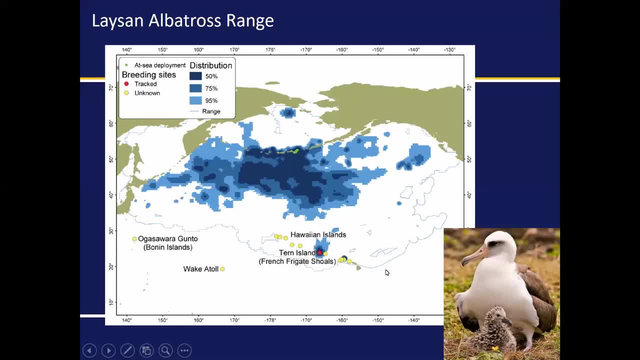 So it is there that they have their eggs and their chick every year, And then they move up into these productive waters of the northern chlorophyll frontal zone where we know there's abundant fish and squid And also lots of fishing activities. So huge range. 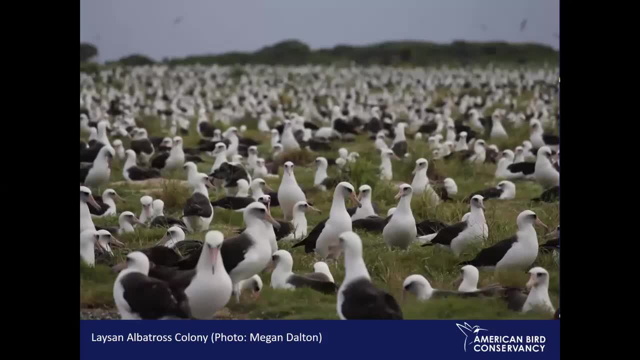 And then they're constrained. They have to come back to these colony areas. So here's a picture of Midway Island mid-season, with lots of activity, And what's quite spectacular to me is that they can traverse these huge ocean basins and then come back to the very same patch of grass on a very particular island. 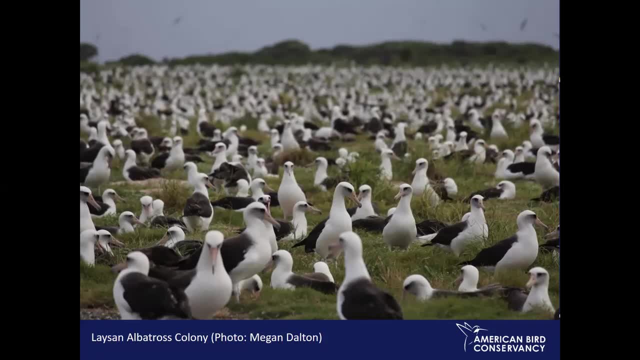 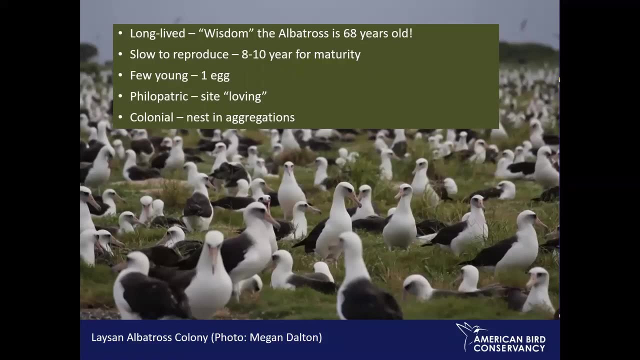 And they will come and wait for their mate, So they're considered monogamous. They're very sight-loving or philopatric and also very tied to their specific mate. So we call these nesting aggregations colonies, And each nest only produces one egg per year. 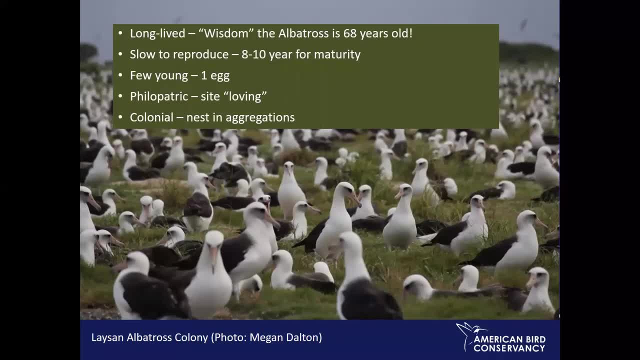 And if they're lucky, that chick will survive to fledging or breeding. But it requires the effort of both parents, And albatross are adapted to make a living in the wide ocean or the pelagic ocean, But it also means that they sometimes have delayed maturity. 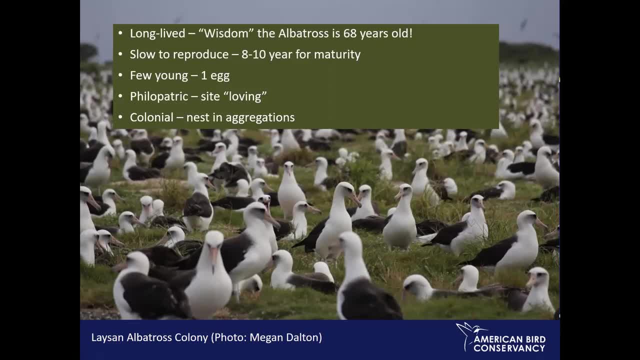 So in many species it's 7 to 12 years. in lace fan albatross It can be as late as 8 to 10 years Until they initiate their first nest, And they're also very long-lived. So wisdom the albatross- it's the, I guess, holds the longevity record for any living wild animal. 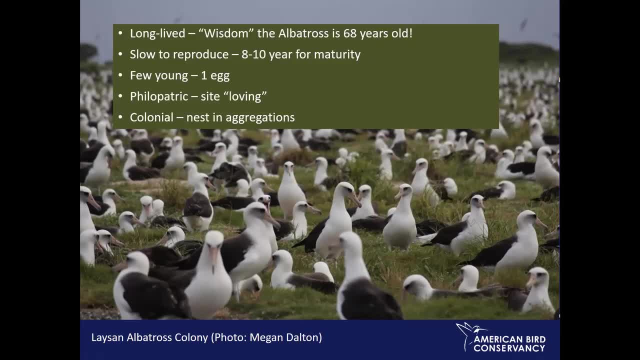 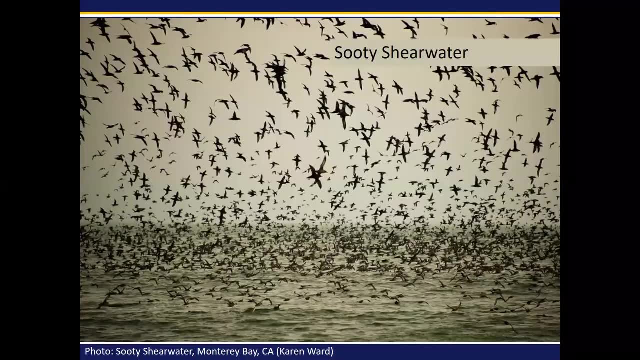 It's 68 years old this year and had a chick, So pretty extreme life history traits. Another species I want to share with you, another one that's in my backyard. This is the sooty shearwater that nests in dense aggregations but also feeds in big dense aggregations. 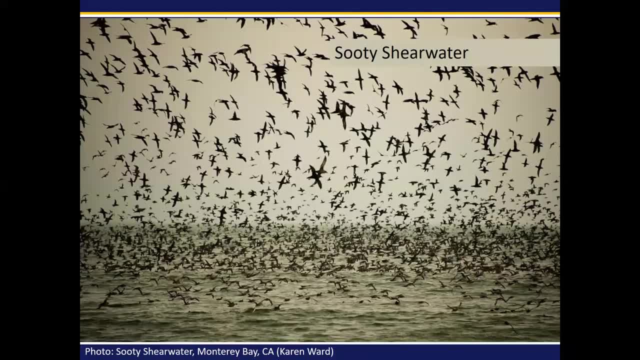 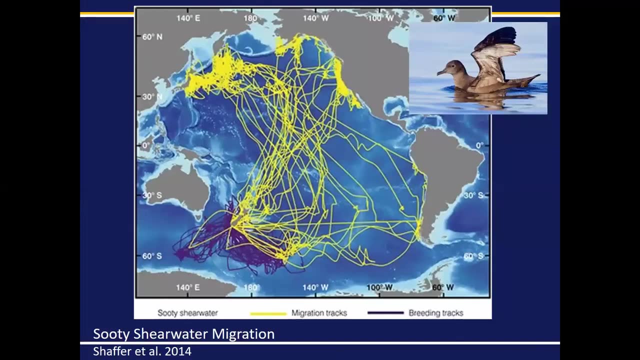 And this is off the coast of Monterey Bay And a picture taken from shore of a huge flock of sooty shearwaters that come into our bay to feed on the great wealth of anchovies that occur every fall. And again, here's the migratory range of these species. 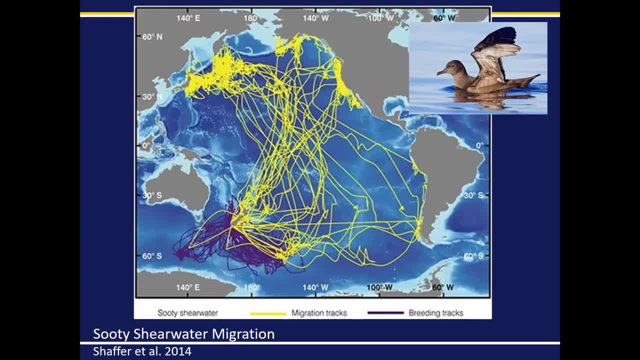 You can see they make these enormous migrations. They have enormous migrations between breeding colonies which are in southern New Zealand up into the North Pacific. And you know this flight from California- I've done it many times- down to southern New Zealand is about 12 hours on a plane. 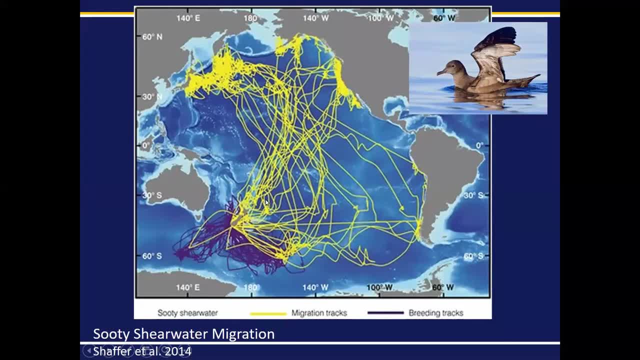 And for a sooty shearwater. it takes about 15 days And they're not really feeding in between the foraging areas in the North Pacific And that transit back to their breeding colony But they're feeding enormously when they reach the productive cold currents of the California Current, the Gulf of Alaska and the Kuroshio Current. 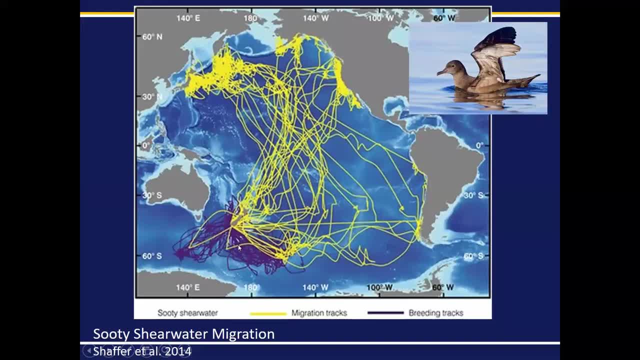 The purple color shows them while they're breeding they're feeding in the Antarctic Convergence Zone. So amazing migratory movements that are very directed. And again you'll get within a nest, one you know: the male going to Japan for non-breeding and the female going to the California Current. 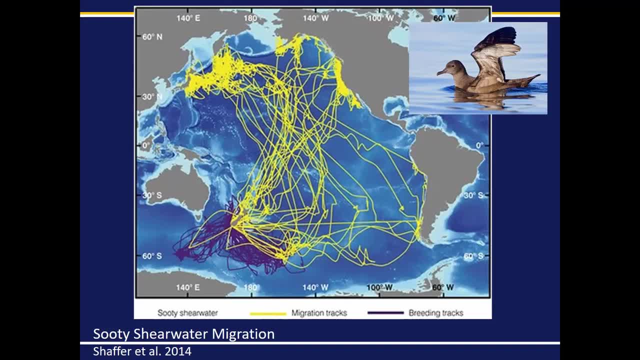 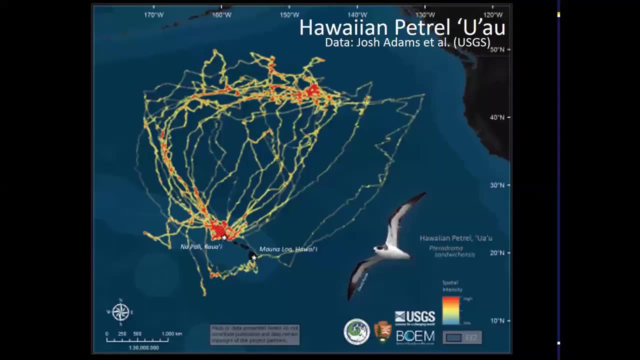 And they return to the very same nesting hole. These guys nest underground every year. So spectacular movements and really critical requirements as far as nesting, So they're concentrated in these nesting areas. So one last example of a far-ranging pelagic zebra. 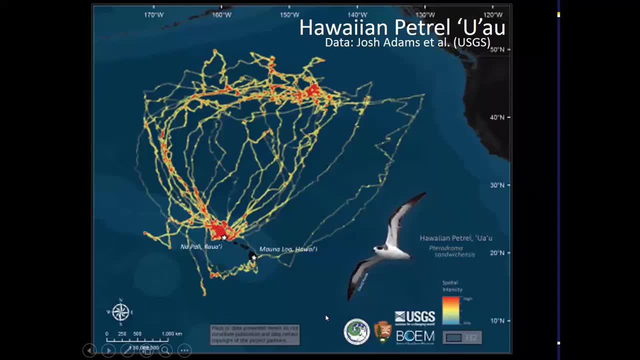 This is the Hawaiian petrel, which is an ESA-listed species that breeds on Kauai Island and Mauna Loa, on Big Island and Maui, And this is data from USGS showing these giant movements that they make from their breeding site all the way up into the Convergence Zone in the Gulf of Alaska. 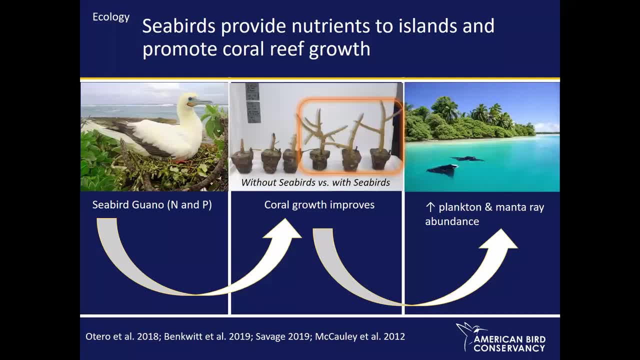 So fantastic movements. They also play important roles in the island ecology in which they inhabit. So this is some really interesting new information that has been published recently, demonstrating that there's a really strong linkage between seabird-derived nutrients and the productivity of the nearshore environment. 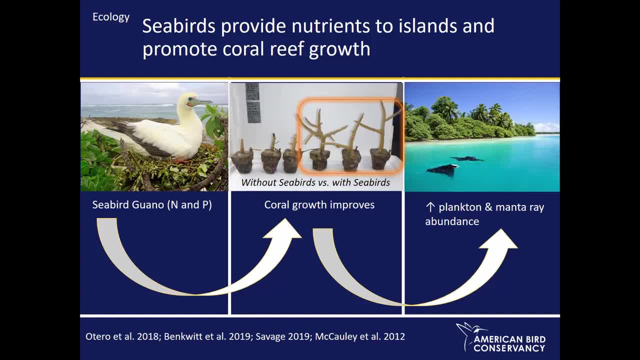 So there's a lot going on here And I'll just quickly walk through. So seabirds- this is a red-footed booby, but I just thought it was a good example of deposit seabird guano in the form of nitrogen and phosphorus into the island system. 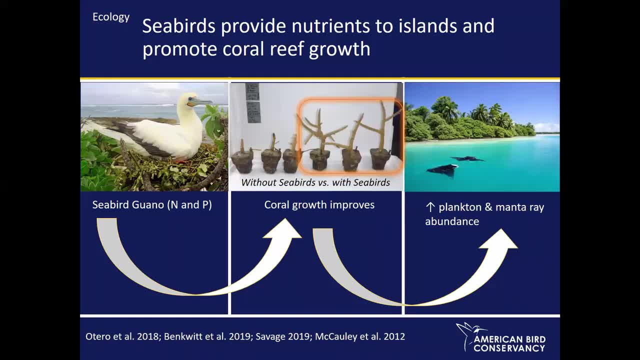 And you can imagine, you know, a colony of 100,000 to 500,000 to a million birds are depositing, excreting great quantities of guano. This gets leached through these porous soils, through rainwater and runoff and into the nearshore environment. 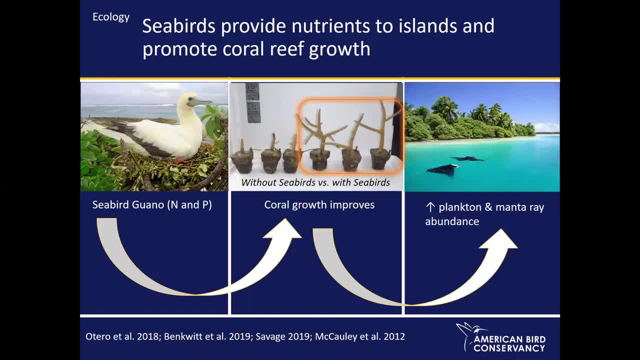 And experimentally people have shown that with the addition of seabird nutrients. so in the middle panel you see improved coral growth compared with treatments where coral propagules are not fertilized with that addition of seabirds. Okay, Thank you. 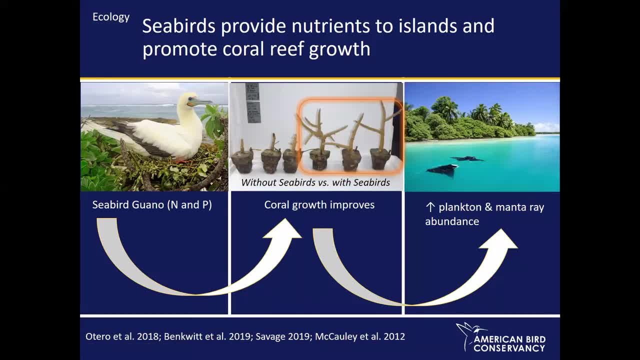 And then here you can see the difference in the amount of nutrients, And so you can see there's a real increase in coral growth as well as a resilience to bleaching, and that was another study that was done. So really interesting, And I put the citations at the bottom and I can provide you with some of those references if you're interested in that. 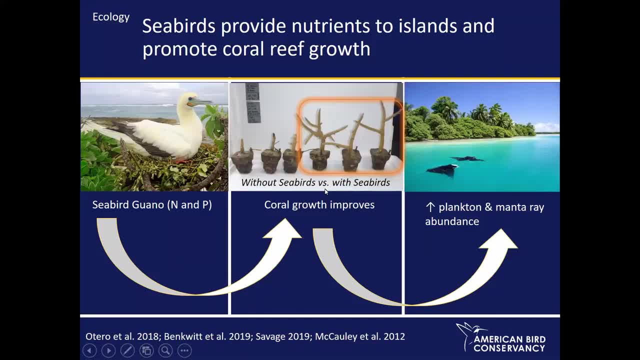 And finally, it not only impacts coral growth but it increases nearshore plankton abundance And this has been shown to increase the abundance of planktivorous fishes such as manta rays, And that study was done on Palmyra Atoll. 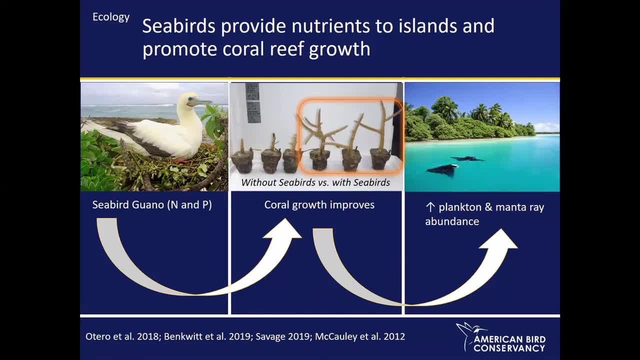 And most of our information comes from tropical islands, which are generally nutrient depleted or lacking in those- nitrogen and phosphorus- But I'm sure that this pattern would hold true as we look at in other areas like temperate zones. So just some of the cool facts about seabirds. 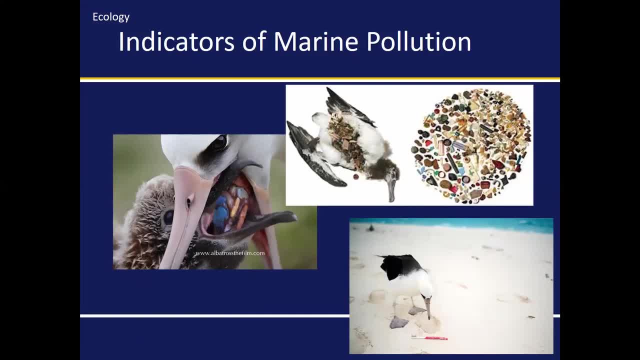 They're also indicators of what's happening in our ocean And many of you have probably seen these images of plastics in albatross chick stomachs And it's certainly a pervasive, ongoing and an increasing threat to these birds And it also indicates pollution. 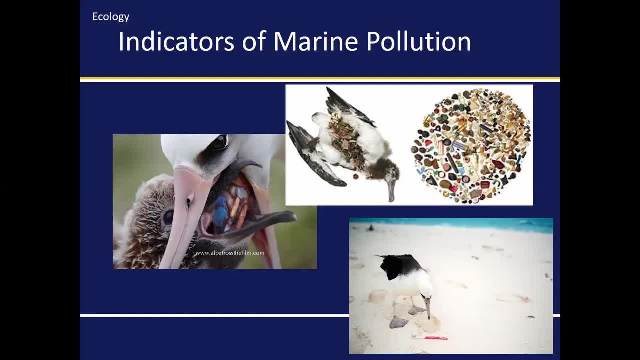 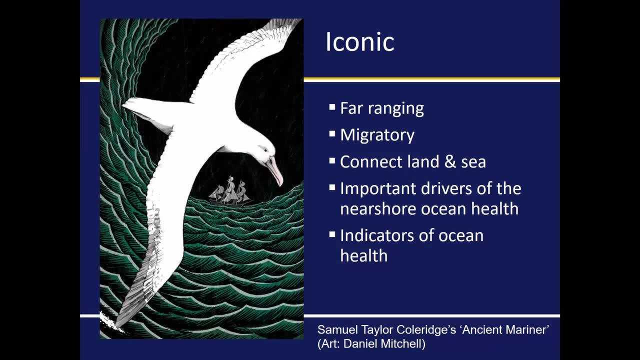 Pollution in our waterways. So I guess the kind of first part of my story is that you know, albatross and petrels and shorewaters are iconic. You know, they're these amazing migratory and far-ranging species that have this ability to connect to land and sea. 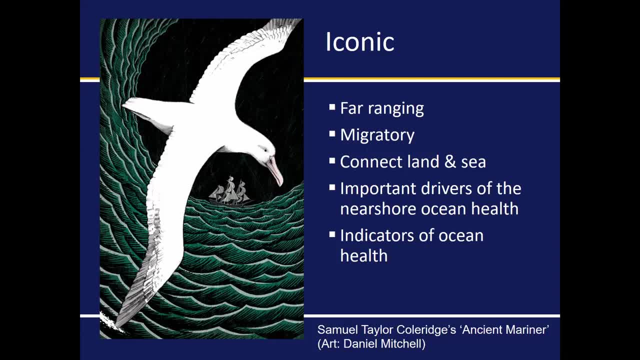 And they are important drivers ecologically in nearshore ocean health and also indicators of ocean health, as we saw with plastics. And they're also really culturally important And there's, you know, the rhyme of the ancient mariner is a classic of you know, connection of people to these wild animals that are out roaming the ocean. 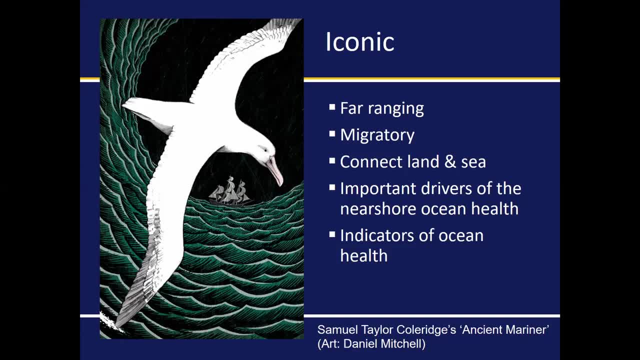 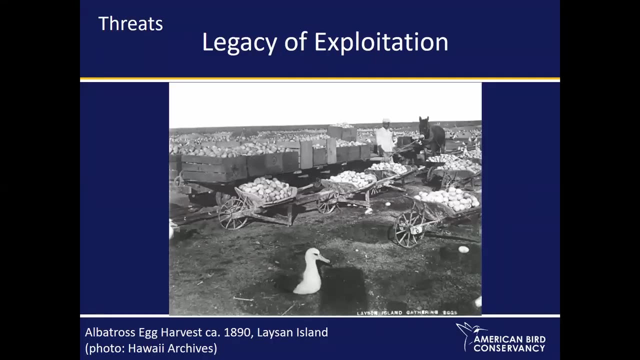 But there's, you know, more recent literature like the Aya, the Albatross by Carl Safina, and cultural linkages with people throughout the Pacific that are really important To recognize as well. So with that I will turn to the threat. 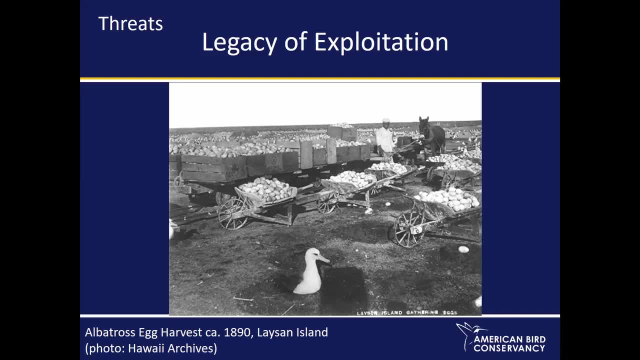 And seabirds, unfortunately, because of their concentrated aggregation, have been subject to a legacy of exploitation, And guano mining on tropical and temperate islands has occurred since the mid-1800s And that also kind of coincided with the extraction of other kinds of seabird parts. 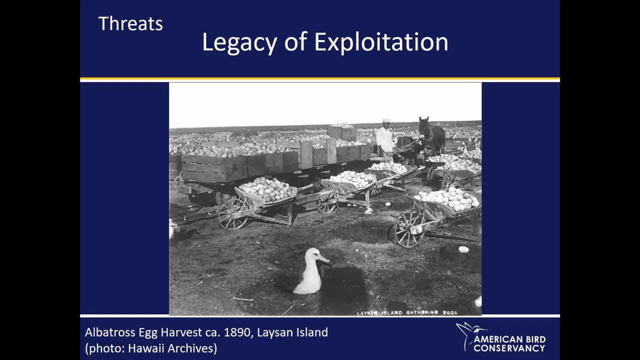 So feathers for the millinery trade and also eggs for human consumption. And so here's a picture of Leysan Island, And these trolleyways were designed for extraction of guano, but they were put to use as well to collect eggs during the breeding season. 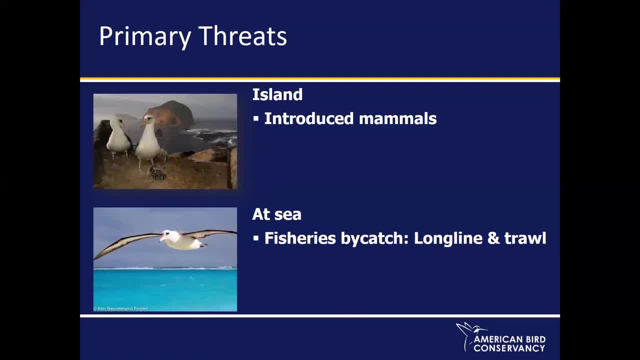 Thank you. Today, the primary threats on islands are introduced mammals, many of which were brought with those early people that came to the islands, Things like rabbits and cats and goats and sheep and pigs. that all decimate these ground nesting seabirds. 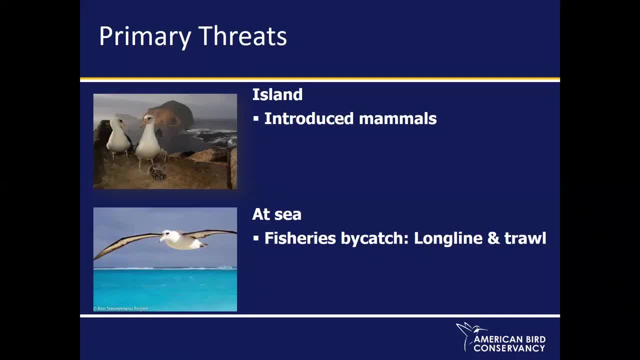 Either by destroying the habitat, as in the case of grazing rabbits and goats, But also direct consumption by cats and pigs. And recently, mammals like mice have been shown to be predators on even the largest albatross, So very vulnerable on islands. 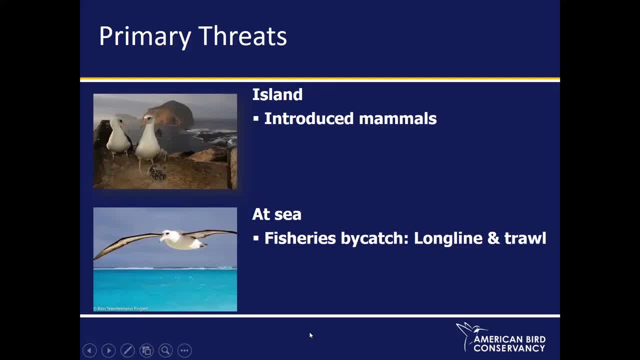 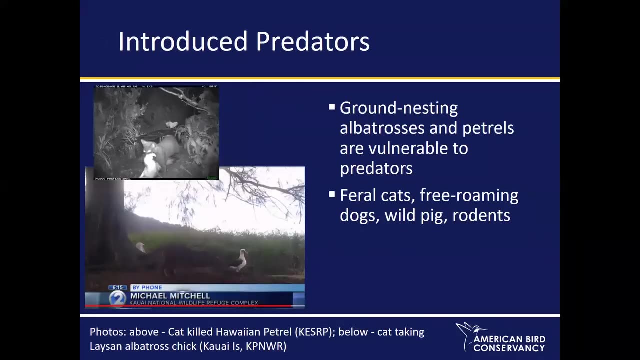 And then at sea, the primary threat is that of fisheries bycatch, And I'll describe that in greater detail, But bycatch in both longline and trout And some other gear types. But those are the primary threats currently, So introduced predators. 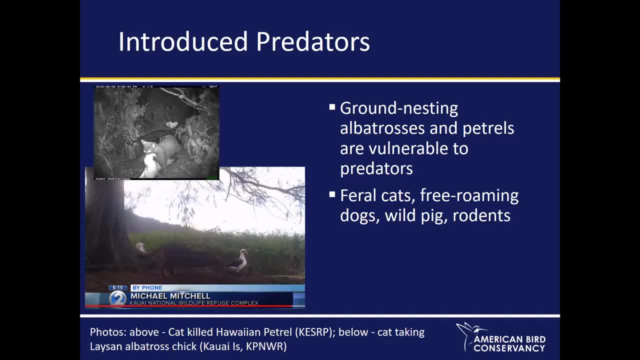 So, as I said, you know, these are ground nesting. albatross and petrels are nesting underground, where they're vulnerable to non-native introduced animals, And these are a couple of screenshots from Kauai Island, where there's a condition, Where there's a continuing issue with free roaming and feral cats. 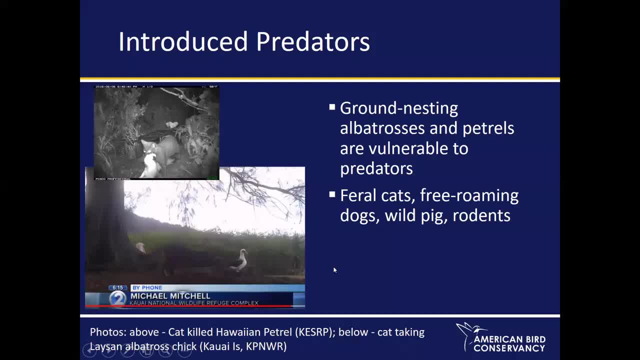 Even coming into National Wildlife Refuge property And they're notoriously difficult to remove. But steps can be taken to protect these colonies. That's introduced predators And ABC has been working with folks to protect some of the nesting sites Around petrels and albatross. 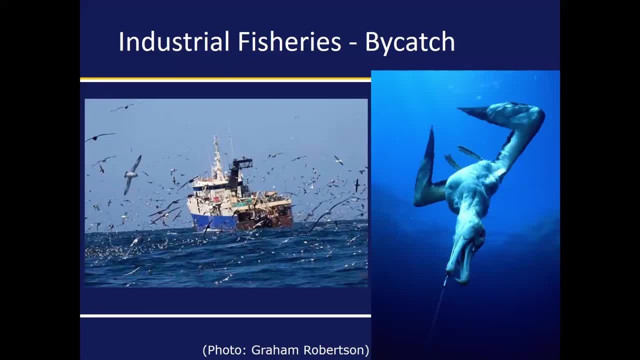 Industrial fisheries bycatch. So bycatch is the incidental capture of birds by fisheries, And ABC started its engagement with fisheries bycatch, as I mentioned before, in the mid-1990s. We helped to draft guidelines for FAO for reducing the incidental bycatch of birds and fisheries. 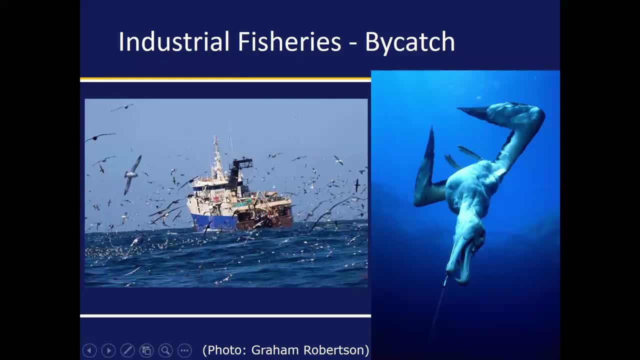 And essentially what we're seeing is that there's an interaction between birds that are attracted by these vessels that are putting out vast quantities of fisheries discards into the sea, And they're also then getting injured by the gear that is deployed from the boat. 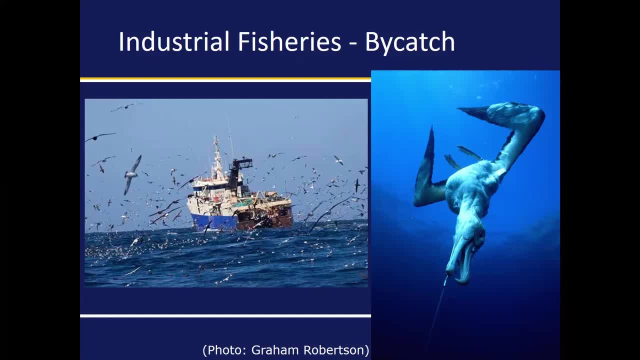 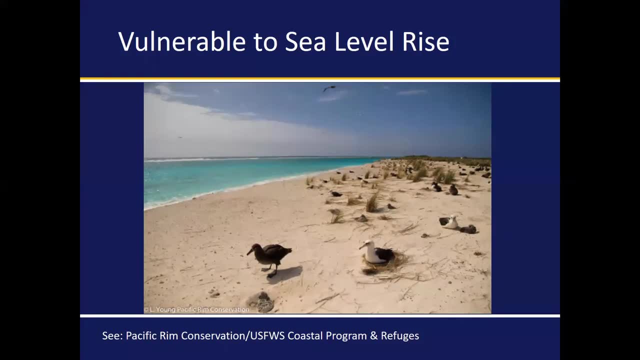 So the baited lines and the hooks, Sea level rise. Sea level rise is an emerging threat, So I put this in here in our threat category And this is particularly an issue for the Hawaiian albatrosses, the Blackfoot and Laysan albatross. 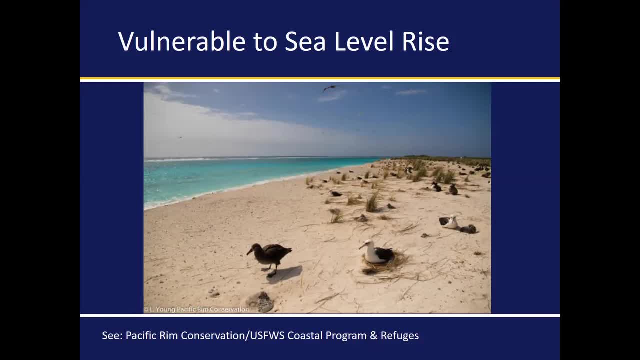 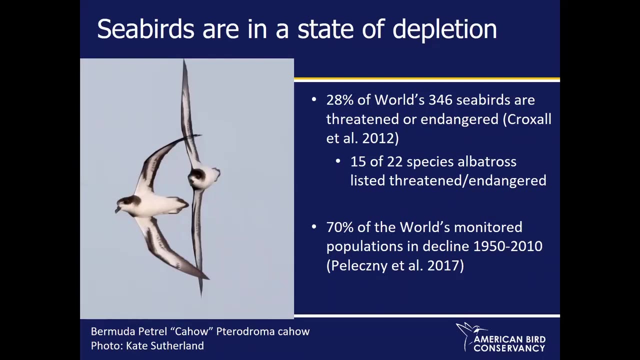 And I would direct you to the Pacific Rim Conservation and Fish and Wildlife Coastal Program and the Refuge Program that's been doing some work to start to plan for that threat. So, as a result of these Primary threats, Seabirds globally are in a state of depletion. 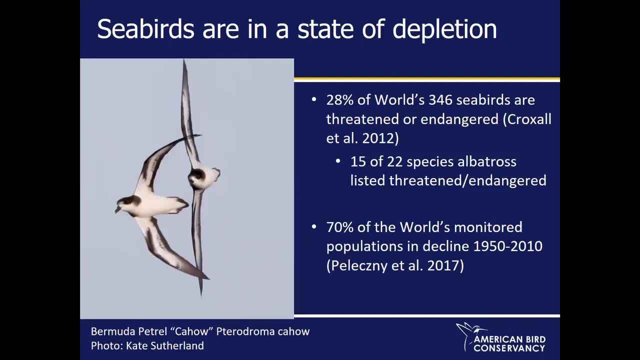 And there's some key papers that have directed our attention to this. you know as early as you know the 80s, But really Croxall's paper in 2012 was a seminal paper to say: look here, a third of the world's seabirds are threatened or endangered. 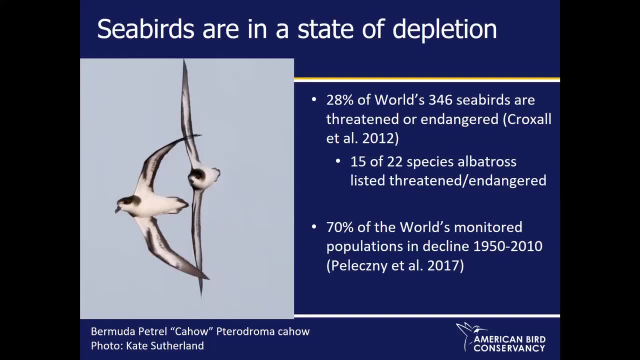 And there's a real need to affect conservation action. So that's what we're doing And we're also looking at the 15 of the 22 species of albatross are listed as threatened or endangered, and we could go down the laundry list of species. 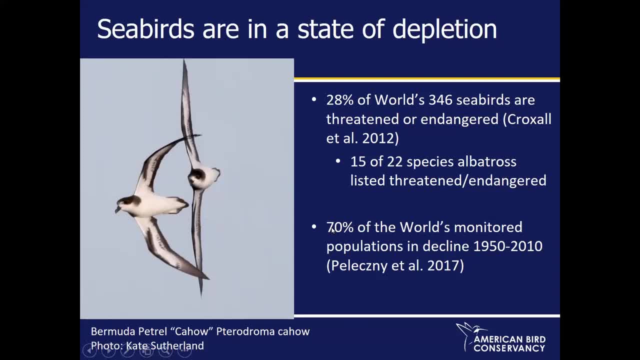 But the threats are pervasive and appear to be increasing. as are these emerging threats, such as climate-induced sea level rise. Polanski's paper that came out a couple of years ago demonstrated that among the world's monitored populations of seabirds- And there's a lot of evidence- 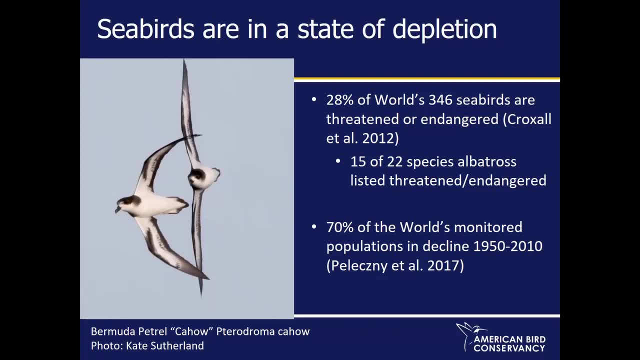 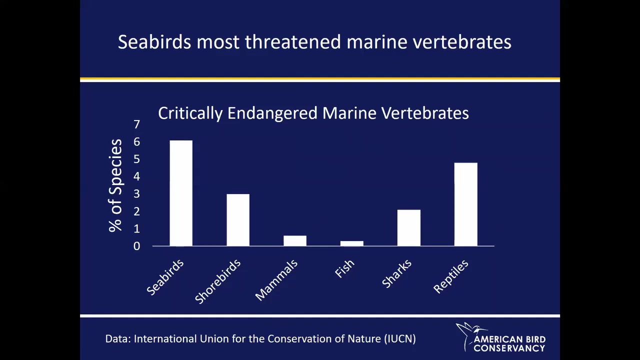 since the 1950s- and this was studies that were compiled of 20 years or more in length- we saw that there's been declines in 70 percent of those studies. so truly, this is a seabird crisis and if we look in comparison to other species of threatened marine vertebrates, so shorebirds 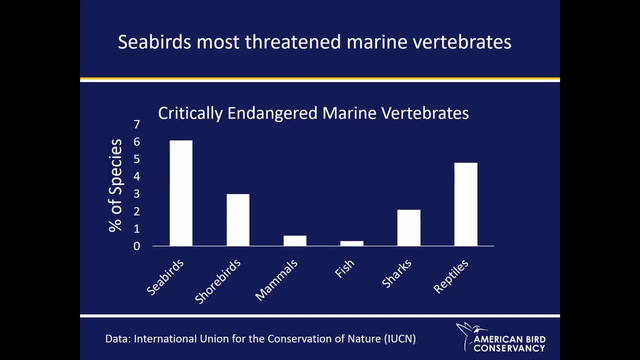 mammals, fish, shark and reptiles. we see that seabirds harbor more of a higher percentage of the critically endangered species and this is relative to the iecm categorization, so they are among the most threatened and we really are at a point where we need to take 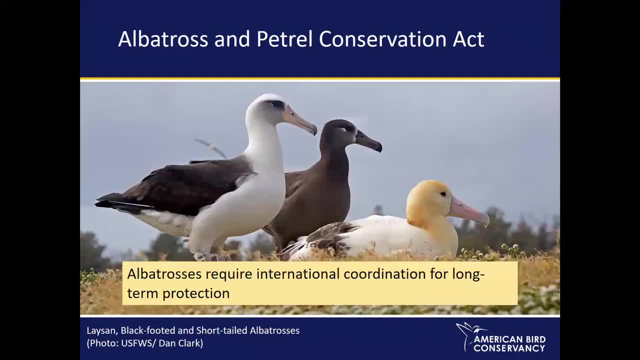 some really coordinated and strong action for these birds. so here the last part of the story is the albatross and petrel conservation act and really in a nutshell, you know to see these birds into the future is going to require a lot of international coordination for the long-term preservation. 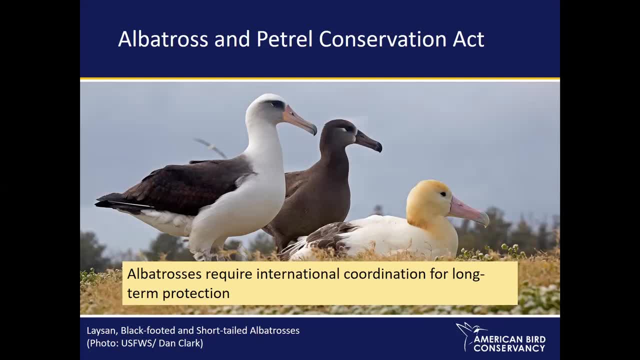 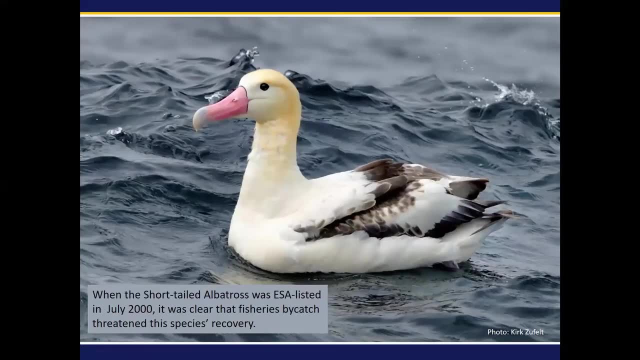 maintenance and enhancement of these populations that have been decimated from the threat. as i said, i've described and i wanted to give you an example of how international coordination can be effective, and this was prior to the advent of the international agreement on the conservation of albatrosses and petrol, or acap as it's known, the short-tailed albatross was listed as an esa. 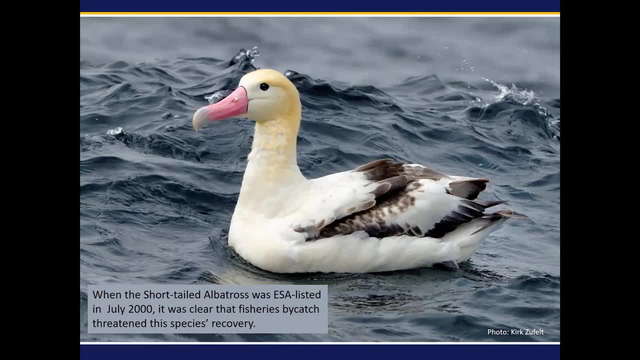 endangered species in july 2000 and it was clear that fisheries bycatch threatened the species recovery and american bird conservancy and other ngos got involved in trying to ring the alarm bells about what was happening with this species and other species in the north pacific and there was a real coordinated action among 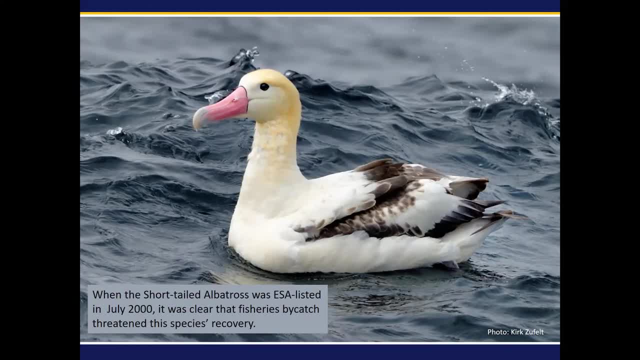 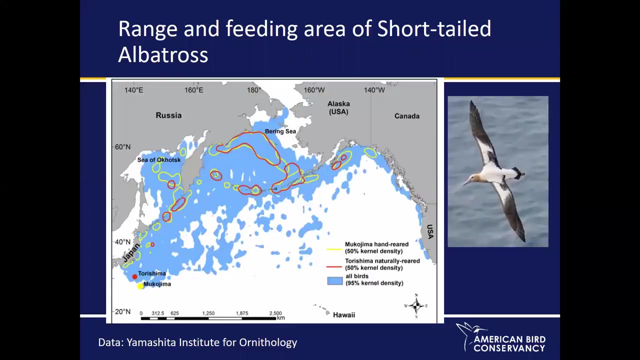 japanese researchers, us fish and wildlife, us mints- and this was sort of under the auspices of esa- demonstrated that recovery and solutions could be found when actions were taken together. So I think it's a really nice example of that. This is the range and feeding area of the. 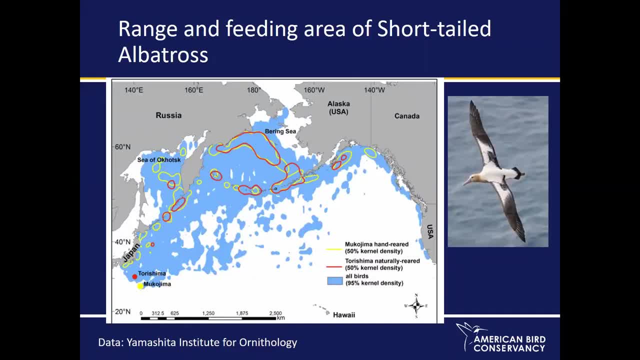 short tailed albatross. So similar to what we saw with lace and albatross, they really traverse the entire North Pacific Basin And these are satellite tracks demonstrating their movement but also the areas of more use in red and yellow And you'll notice off the US coast you'll see also 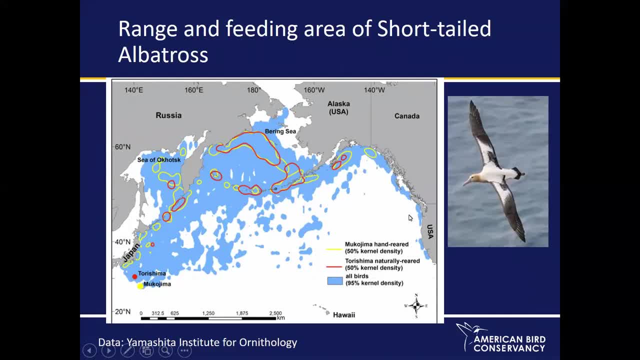 these little blobs, and we've recognized that the coastal waters are really important, including through the Bering Sea, there's this shelf break area that's very important for this species, And so, in addition to satellite telemetry, to understand where these birds were traveling to, what the range overlap was, 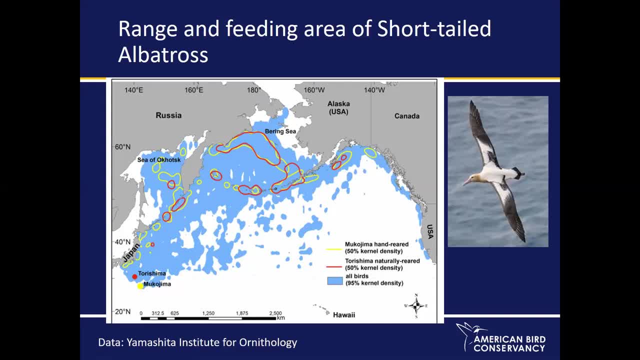 there was work done on the colonies, colony restoration, protection and transportation to enhance those populations, And then there's quite a bit of work in fisheries on mitigation, And so in the end we're now looking at the short tailed albatross And we're seeing 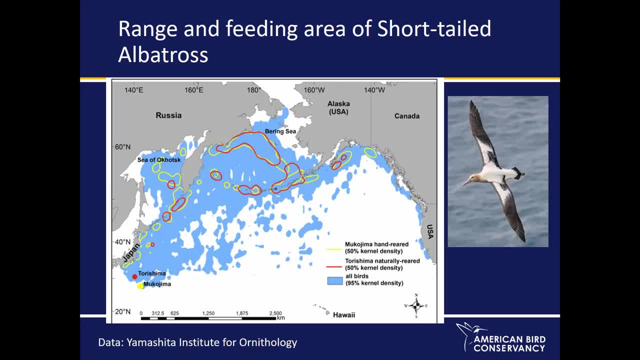 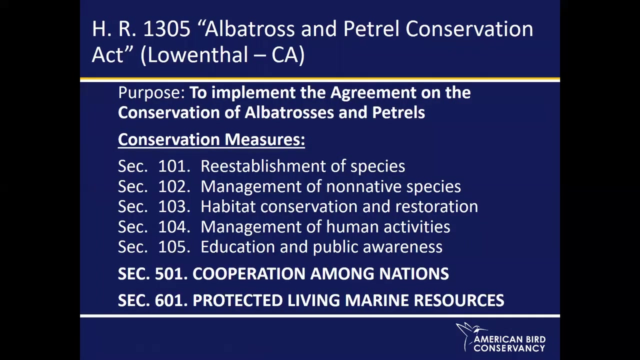 that the short tailed albatross is increasing and expected to do so into the future, And it is that international collaboration, among an interagency collaboration that's helped to promote this species. So I think this is a great case example of how what ACAP is doing will benefit these birds. So then, 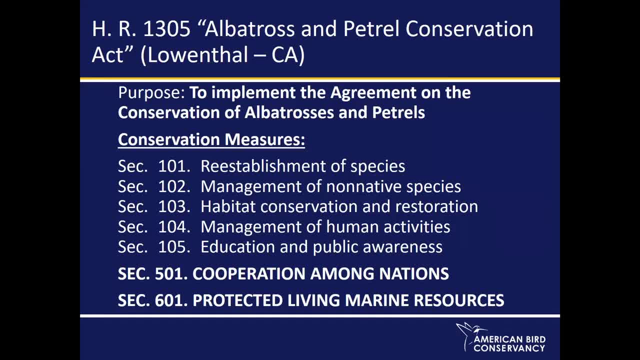 let's talk about some of the other things that we've talked about, some of the nitty gritty. So this bill that's been introduced- HR 1305, Albatross and Petrol Conservation Act- by Senator Lowenthal from California- is really the purpose. 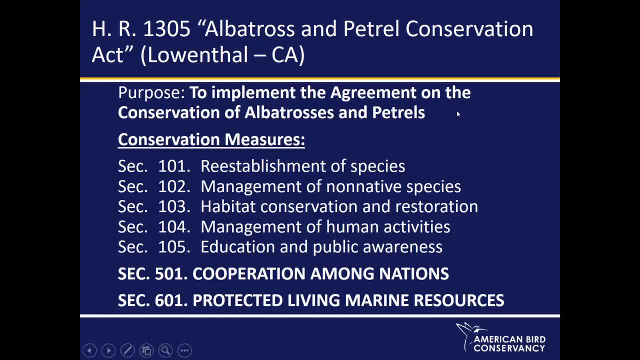 of this agreement is to implement this larger international treaty called the Agreement on the Conservation of Albatrosses and Petrels, And that agreement is signed by 13 party states, including many uh range states in south america and the southern hemisphere, and mexico, canada, the us and at times, japan have all participated in meetings of acap as range. 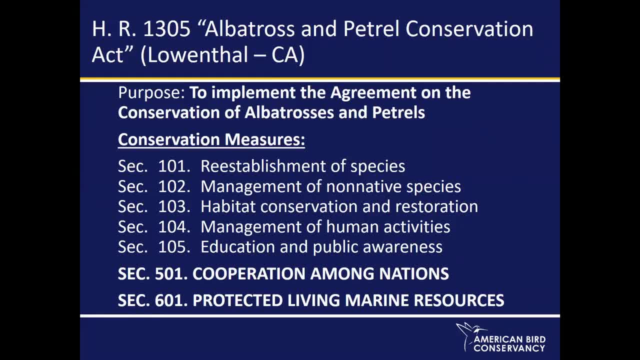 state non-party range state members. so we already have spent a lot of effort having people attend these meetings and participate as range state members, but this act in the us has passed would allow us to become more formal decision makers and to more fully implement some of the conservation measures. 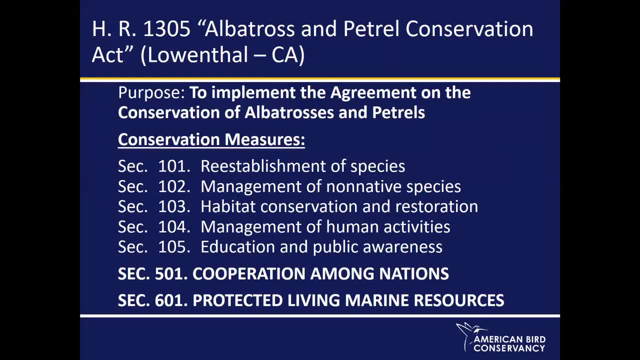 that are outlined and i grabbed from the text of the bill. the conservation measures that are outlined, including the re-establishment of species, as we've seen with short-tailed albatross, was a really important part of the recovery efforts for that species. management of non-native species habitat and conservation and restoration actions. management of disturbance. 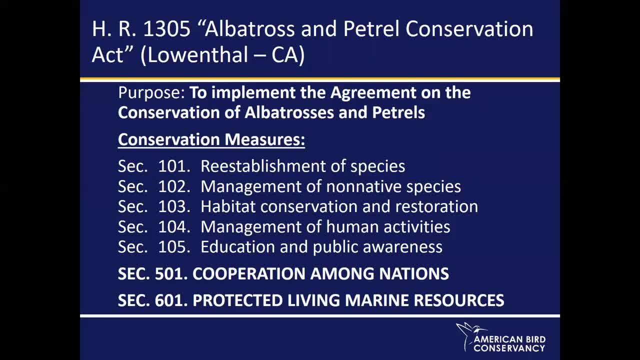 and other human activities, as well as education and public awareness, and another key part of this is that interaction and coordination among nations. and so if you reflect back on that albatross range map, you know those birds are traversing the entire pacific basin, so the cumulative impact of fisheries need to be determined. 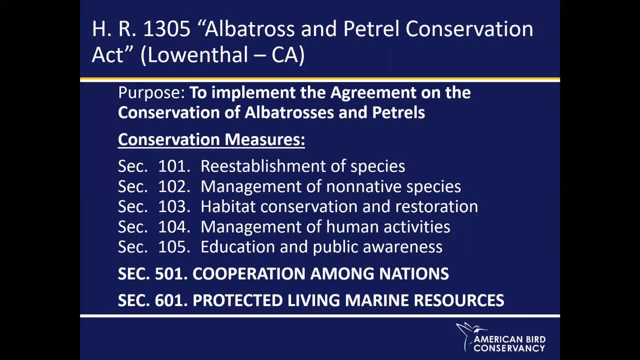 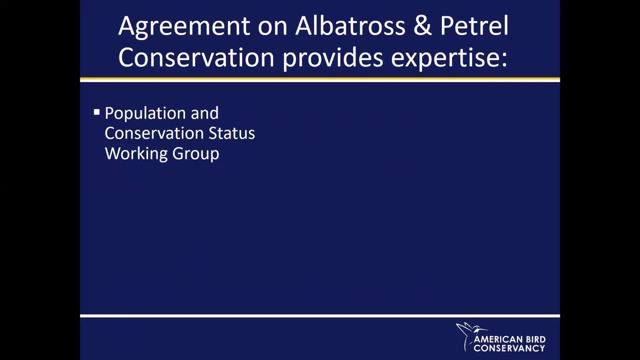 as we start going forward with the conservation of these species. um, how does acap affect change? and i've been fortunate enough to attend two of these acap meetings. they occur every about 18 months. the working group and the advisory committee meets every three years and really the nitty-gritty of the work goes on in the working. 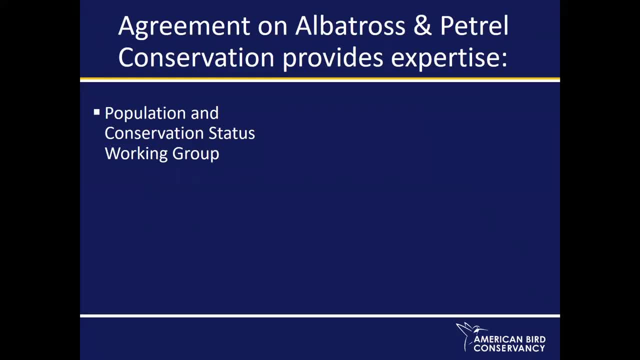 groups, and the two main working groups are the population conservation status working group, um, and also the seabird bycatch working group, um. and so if the us were to become a party, we'd have more of a voice and influence within these working groups and be able to bring our expertise and 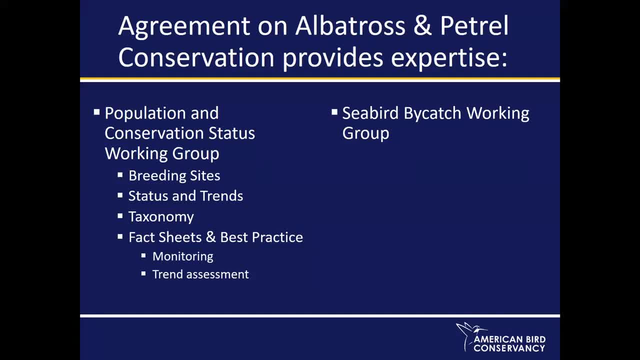 share our information on the status of our species, the trends that are happening and help craft act sheets and best practices for monitoring and trends assessment. and that's a really important part of the work of the population working group, the feeder bycatch working group is. it is an interesting place where a lot of technical expertise is shared. 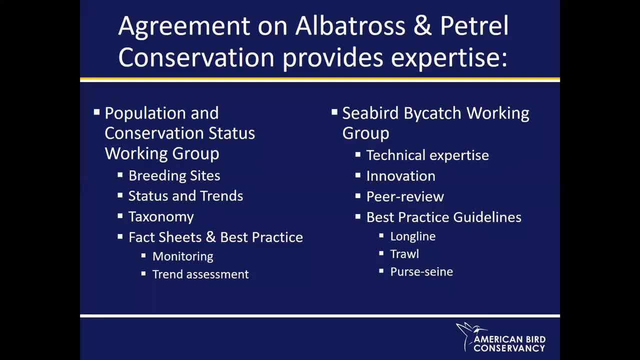 and innovation, innovative solutions are crafted, and i should say here that interacting with the fishing community has been a really strong component of the work of the bycatch working group. so many of the experts work directly with fishers to design solutions for reducing bycatch. the process is peer-reviewed. 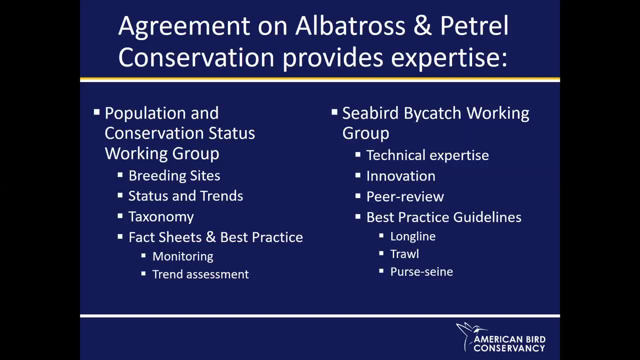 so there's white papers that are presented and everybody has a chance to review them and vet them, and it culminates in best practice guidelines that are put in both technical terms and lay terms, specifically for the most damaging fisheries for these birds, so long line trawl, and they're also 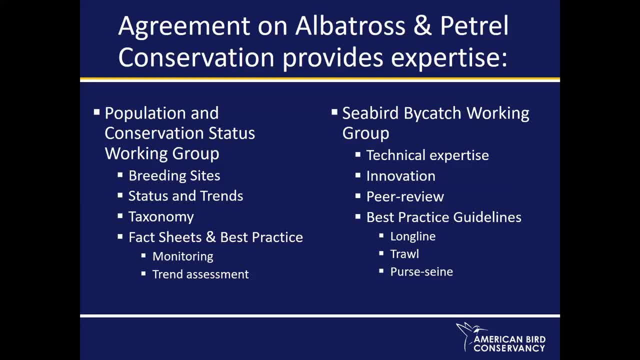 drafting guidelines for per se fisheries, and a key part of this is it's all voluntary in terms of the the guidelines. these aren't mandatory guidelines. these are demonstrated and they're not mandatory guidelines, so it's all voluntary. it's a demonstrated best practice with a high level of rigor, and so the technical advisory group is putting the information out there for the nations and the party states to review and to use as they see necessary to protect the birds in their waters. 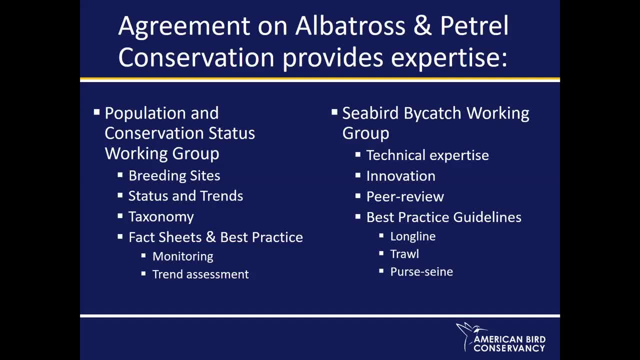 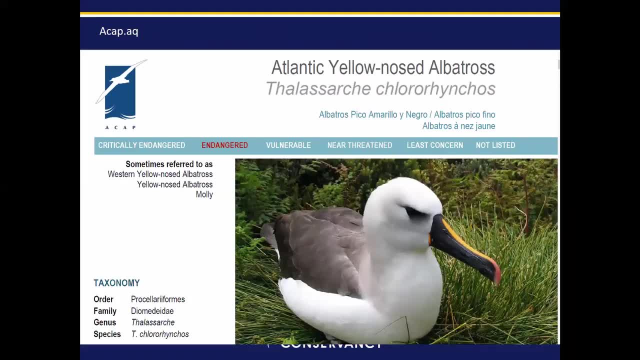 and so there's no enforcement that's enacted through this treaty. here is an example of a fact sheet, and so you can go. the website is acapbitaq and you can look up all the species that are listed. currently, there's 31 species listed under annex1. 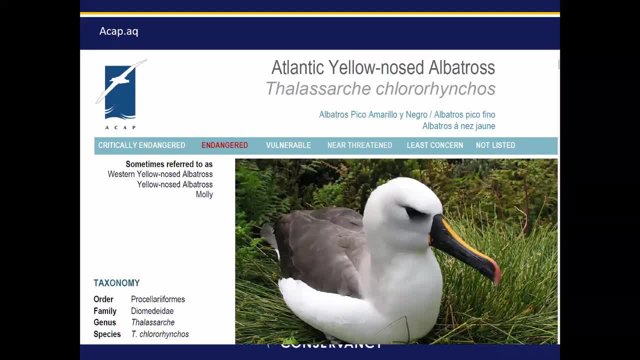 this includes all of the large albatross, all 22 species of albatross, two species of petrels and seven cheerwaters. so quite a diversity of birds. but you can look at the fact sheet and get a synopsis of the status, the conservation needs, the threat and the current action. So they're providing very 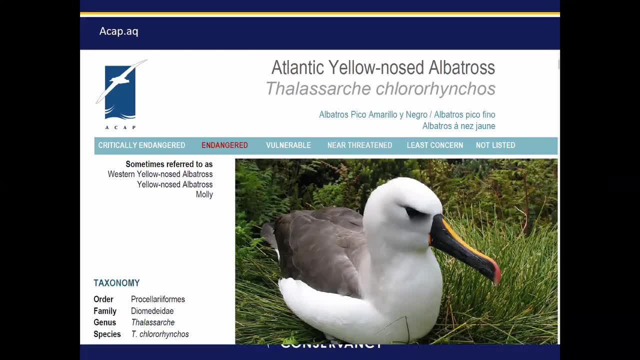 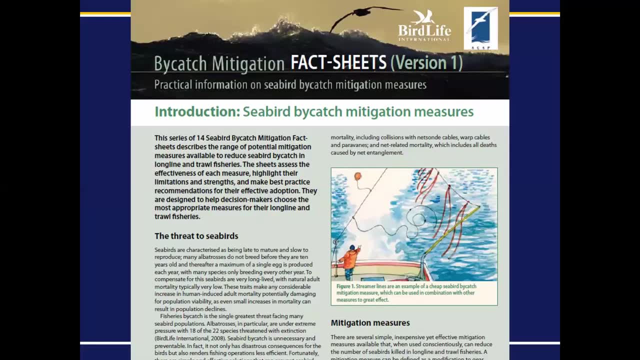 tangible, hands-on information that's freely available, So really important resource. And then they also provide these mitigation fact sheets. So here is an introduction to the Seabird Bycatch Mitigation Measures and there's a series of 14 fact sheets. 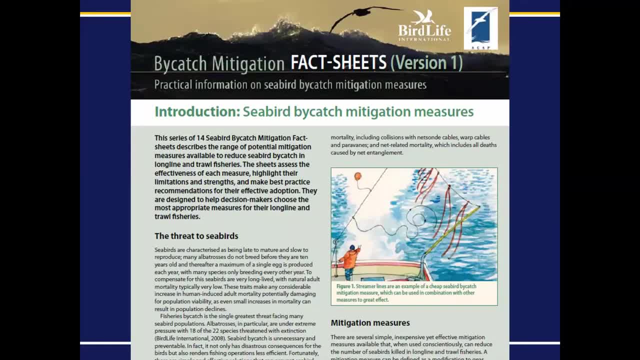 that demonstrate what types of mitigation are possible for different fishery types and how they've been implemented, And they also provide the technical references for people that are interested. So really important resources that can be made use of by governments of both participants in the treaty and non-participants. So this is not a 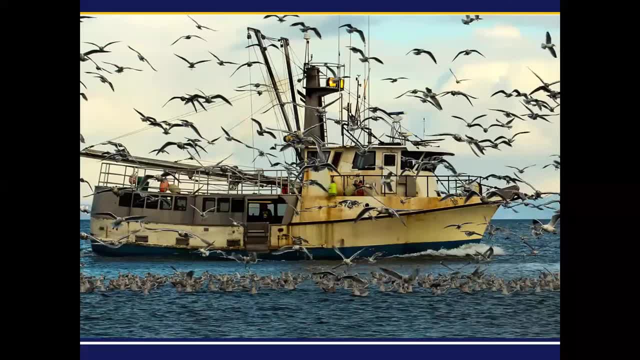 closed process at all, and that's sort of the beauty of it. So how does this work? I thought it'd be a good example. So, in practice, academics and researchers go out and work with fisheries, where they know there's an issue and a problem, and they bring 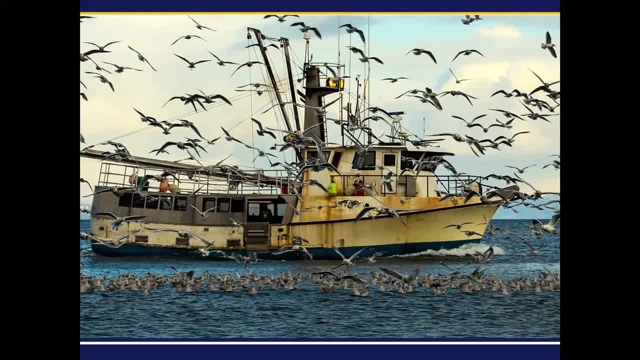 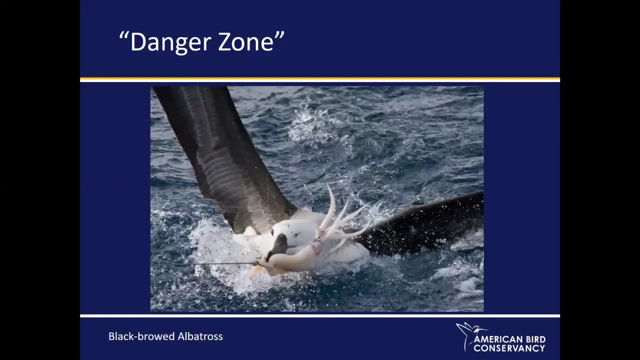 their innovative solutions. And then they also provide the technical references for these facts. solutions back to the table, to these working groups, in this case the seabird bycatch working group. We know there's this area of fisheries behind the fishing vessel. that's sort of the danger. 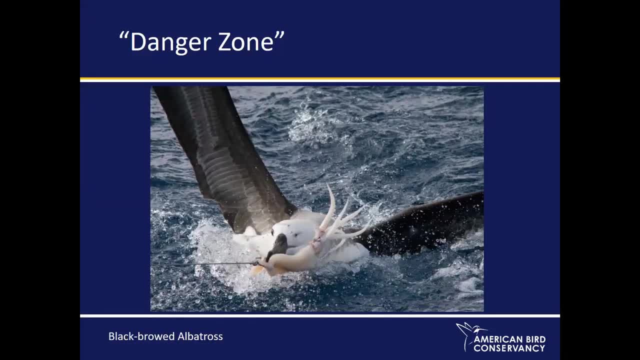 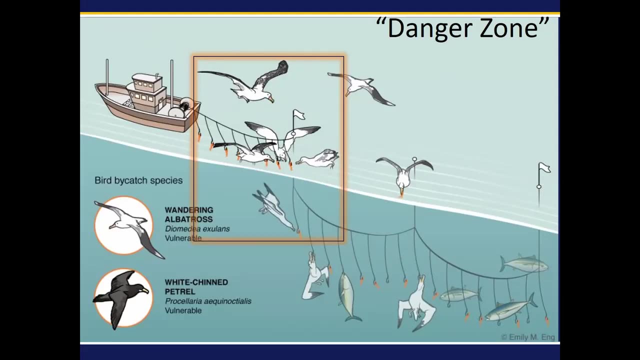 zone. So birds can either get, for example, caught, as the target fish is being recovered, on the haul, or on the set, as it's going out. And here's the danger zone behind the vessel in the schematic that I pulled from BirdLife: 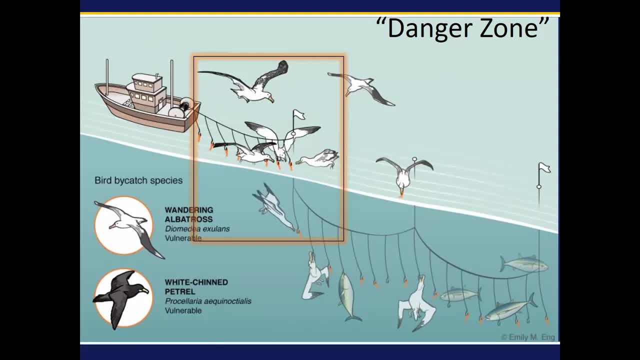 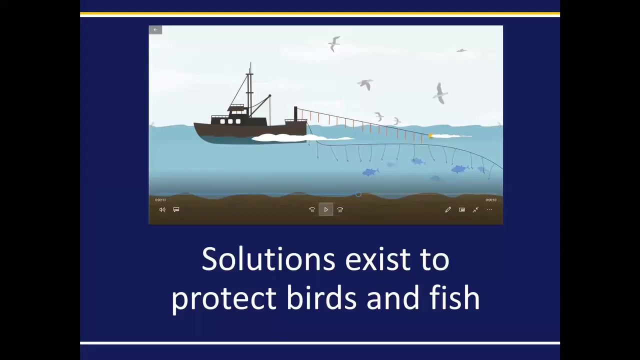 And you can see that it's really in this one concentrated area. So there's been some interesting developments in terms of mitigation for bird interactions in this zone, most recently things like hook pods, But the most tried and true are things that are really basic. 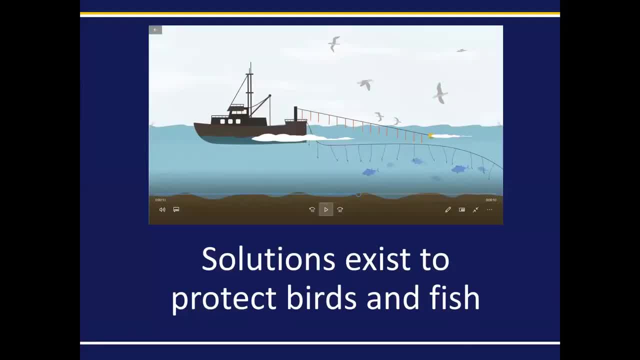 These are these tori lines, or streamer lines, and this is a schematic showing this bird stream line that goes back beyond the back of the vessel as the hooks and lines are being deployed. And if you look at the American Bird Conservancy YouTube channel and search for bycatch, we 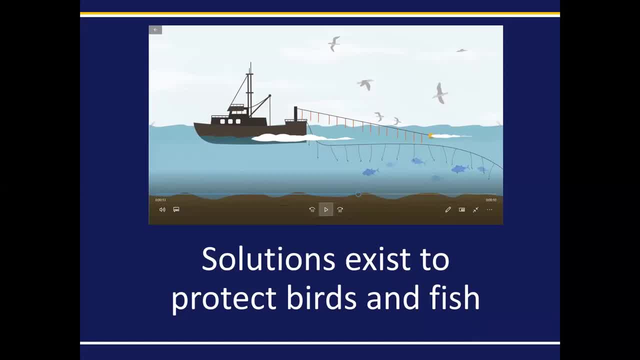 have a suite of videos that we produce in English and Spanish to describe the nature of interactions with different types of fisheries And some of the mitigation that is effective in those fisheries. So solutions exist, but we're in a constant state of finding new innovative solutions. 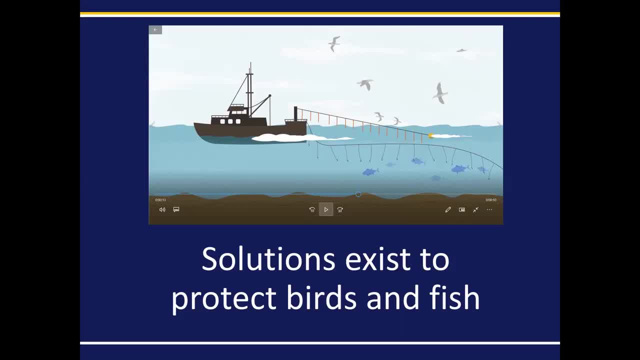 that are technically practical and also very cost effective. So those are some of the criteria that the bycatch working group looks at when they want to advise on a best practice, because you may design the you know most efficient, effective mitigation measure, but if it costs $300 a piece, it's not going to be practical. 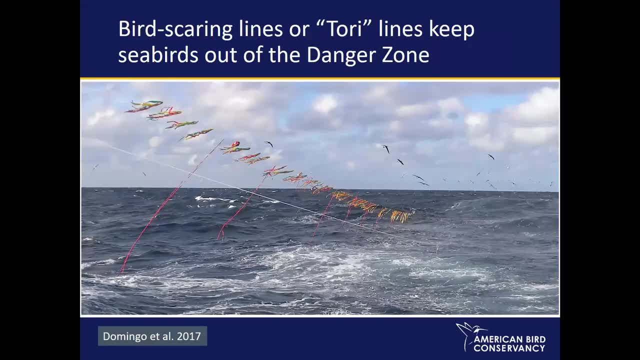 for those fishers. So here's an example of bird scaring lines, or tori lines as they're known, to keep cedars out of this danger zone, And this is one of the ACAP best practice efforts, And it not only protects lines like long lines that are going out, but it can also be effective. 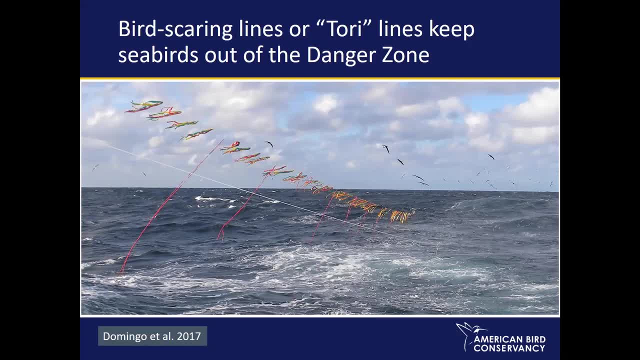 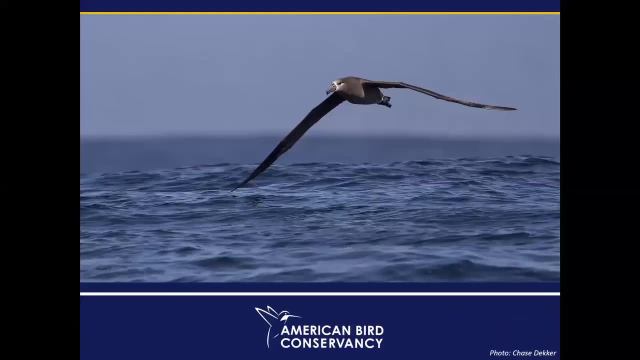 in trawl fisheries Where there's a third wire or net phone cable that's tracking the net and going down. So this is a real efficient way And, as a result of using this mitigation, a recent analysis. sorry, we'll go on to the 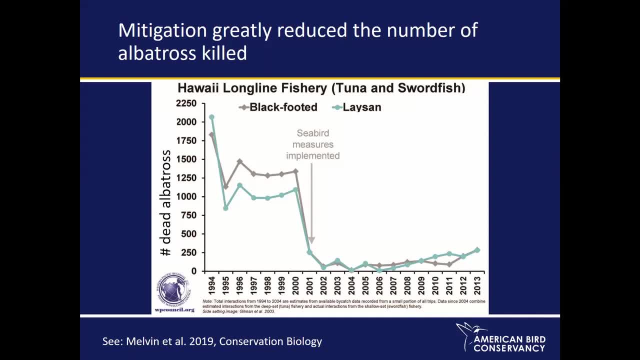 next slide has shown that in the US fleets where these mitigation efforts have been put into use, We've seen a dramatic increase in net phone cable. So this is a real efficient way And as a result of using this mitigation, a recent analysis has shown that in the US 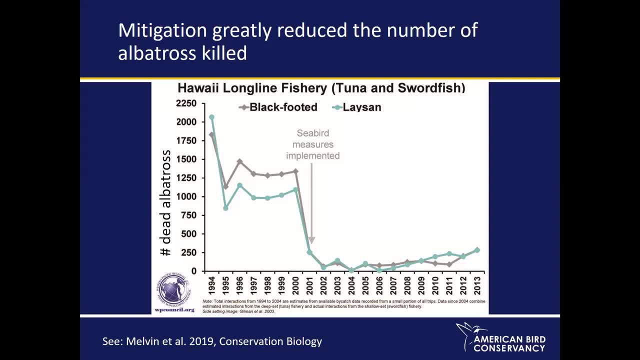 fleets where these mitigation efforts have been put into use, We've seen a dramatic decrease in the numbers of albatross killed in these fisheries. So this data is from the Western Pacific Region and Fishery Management Council, But there's a more recent paper by Ed Melvin looking across four different fisheries in Alaska. 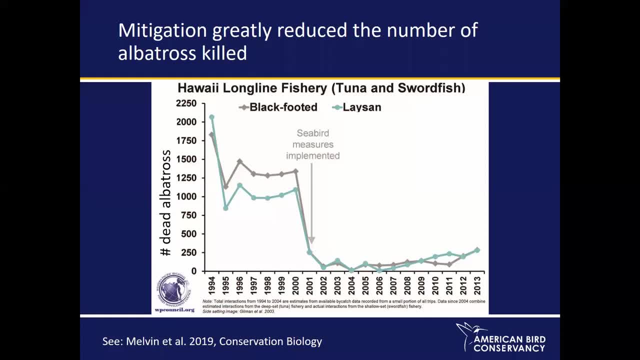 demonstrating the same thing where bird catches go down dramatically, when simple mitigation such as tori lines or tori lines are being used. tori line or bird streamer lines are put into use, and this is the kind of information that's really important in demonstrating those best practices that it it can be effective in reducing the number. 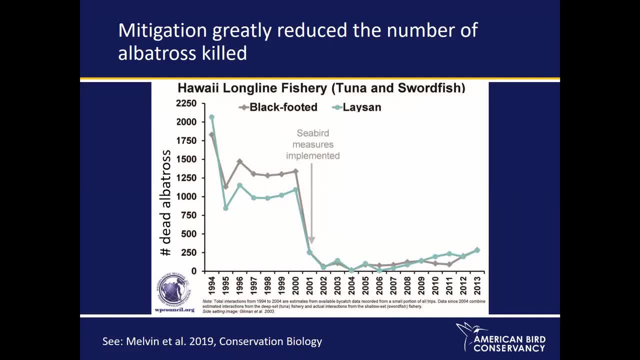 of albatross, and then also another criteria is that it doesn't decrease the target catch for the fishers, because again, that's going to be a no starter if you're decreasing the non-targets. so many of these seabird measures were implemented in response to the heavy bycatch of our north. 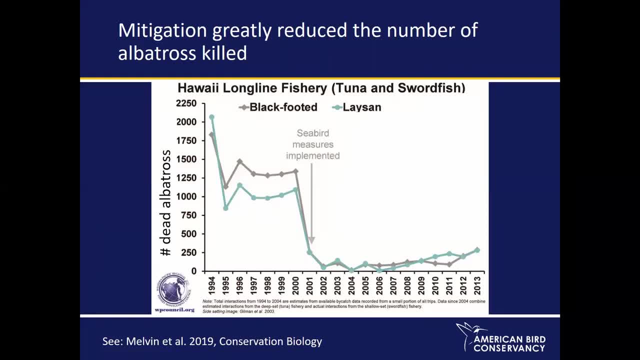 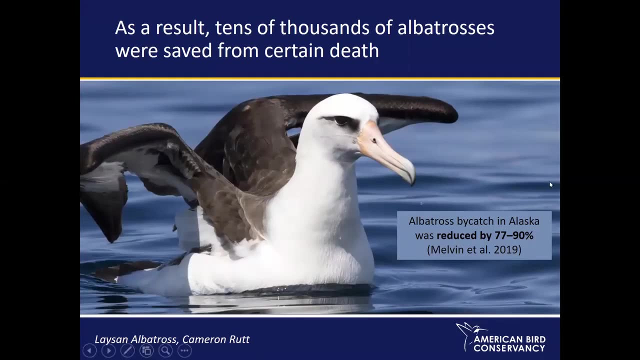 pacific species and so in the us waters many of the mitigation is already being that's advised by acap is already being implemented in our fishery and here's the annotation here: in alaskan fishery they were already reduced: albatross bycatch, both lace and- and blackfoot, 77 to 90 percent in the four fisheries. 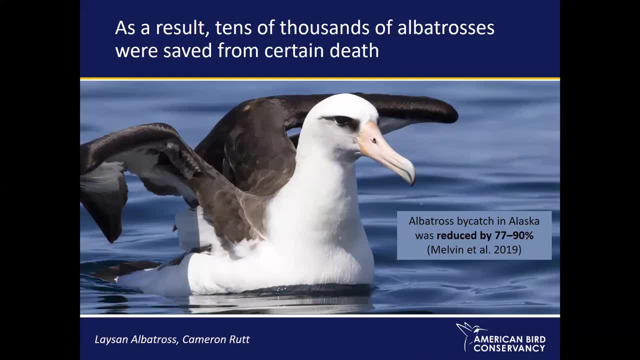 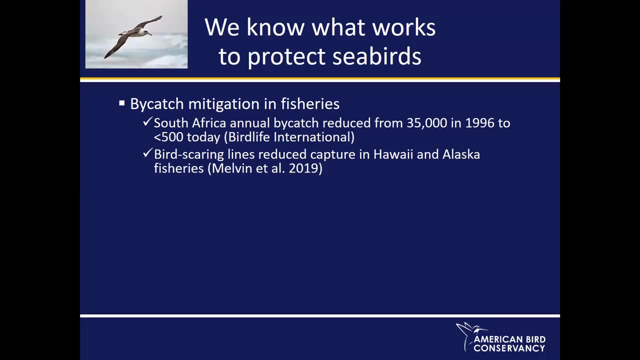 that they looked at after the implementation of mitigation. so we know that it works and that tens of thousands of albatross can be saved by implementing this, these mitigation measures. so we know it works and bird life has demonstrated this in other places like south africa and, as i mentioned, they're constantly looking at new innovative tools, such as hook pods. 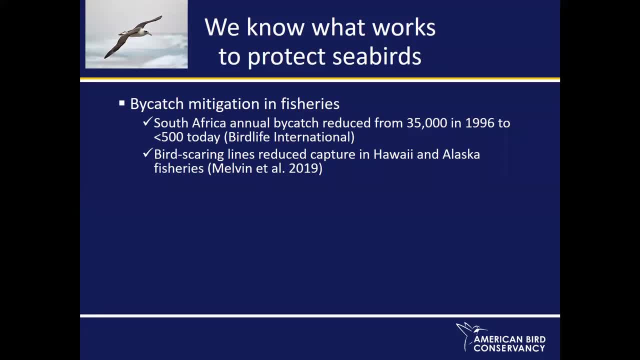 but simple methods such as bird scaring lines and the timing of setting has also worked to reduce bycatch. we also know that removing threats on islands works to increase the number of birds and provide resiliency to these populations that i didn't have time to go into great detail about efforts on seabird breeding islands, but 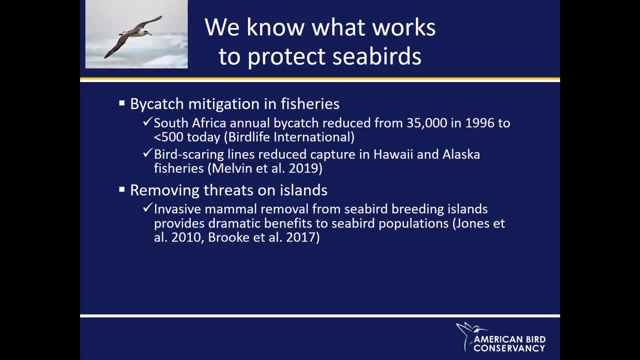 the jones paper and brooks paper cover some of the dramatic benefits that we see from the removal of non-natives. and then, finally, you know, international coordination is essential for this conservation across the range of the pelagic species. and, unfortunately, spending a lot of time in rooms. 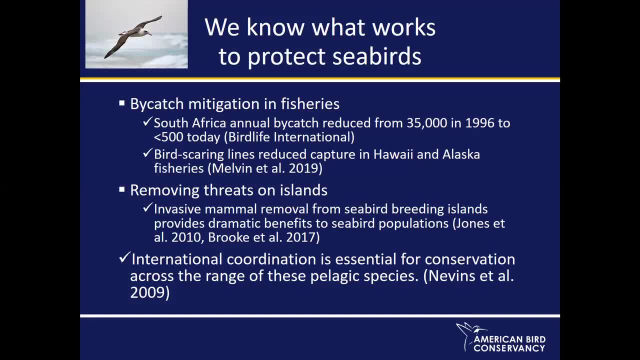 species and their concerns is a big part of our jobs as conservationists and managers. to plan for the future and also to try to figure out what, which actions will be the best use of our funds and how we can leverage change across the range of the species. 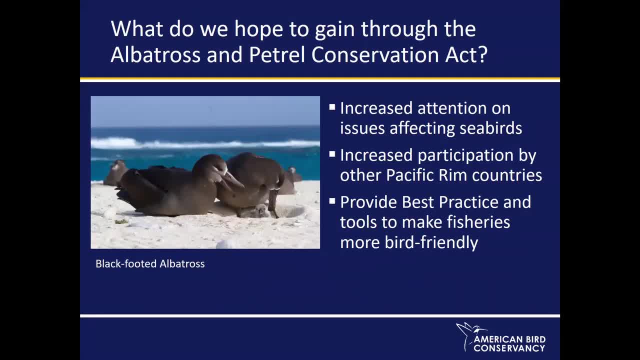 so what do we hope to gain through the US's accession to ACAP and the passing of the albatross and petrel conservation act? we hope that we can increase attention on the issues affecting seabirds and now that I've given you sort of a seabird 101, hopefully you have more. 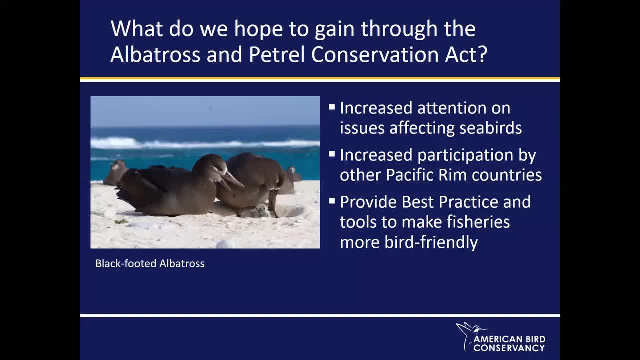 information or know where to look for information about the threats that are impacting the seabirds and the solutions that are out there. we hope by the US participating in this international treaty we'll have other pacific rim countries participate, our neighbors to the north and south. 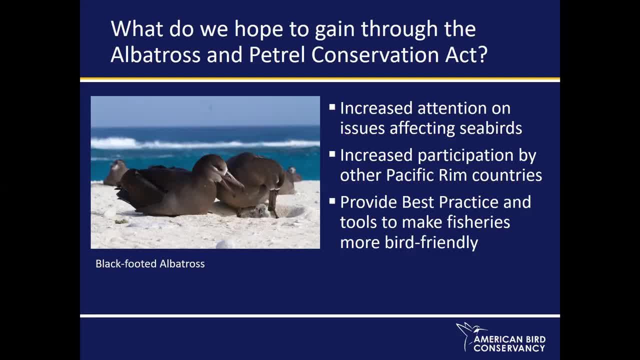 Canada and Mexico, as I said, do participate in the ACAP meetings, although they're, like the US, non-voting members, and so we may help to leverage their participation, and I hope that we can continue to do that, and also we can provide best practice and tools to make. 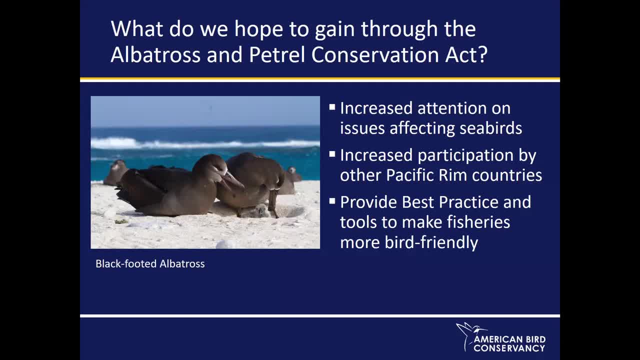 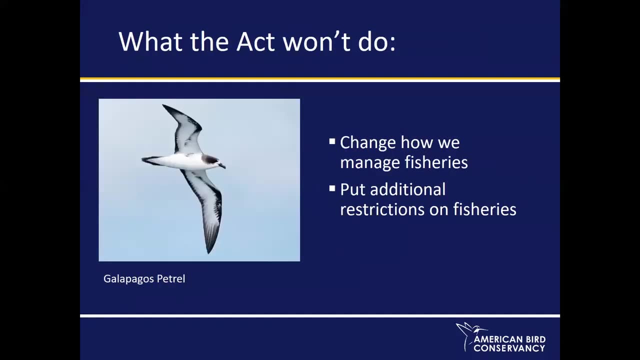 fisheries more bird friendly, not just in the US, where many of these mitigation measures are already in place, but to kind of level the playing field across fisheries globally and bring them up to the standards that we already see. what the act won't do- and I think this is important to cover as well- it won't really change. how the act is going to be implemented in the US, and I think this is important to cover as well. it won't really change how the act will be implemented in the US- and I think this is important to cover as well. it won't really change how. 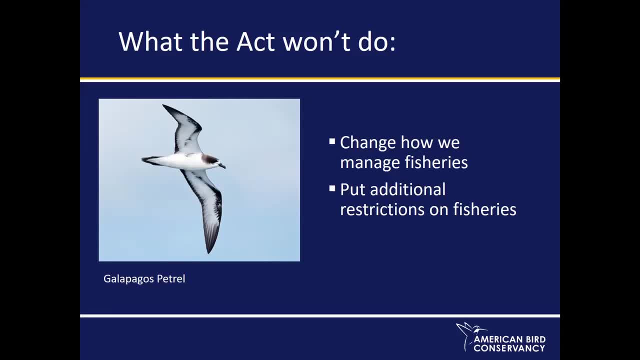 we manage fisheries. as I said, there's no enforcement changes to the level of enforcement and it won't put additional restrictions on fisheries. it'll just provide tools and expertise so that fishers can become more bird friendly. and, as you know, the seafood market is coming under increasingly.